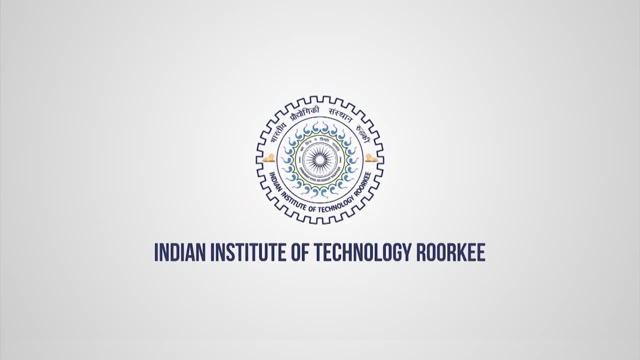 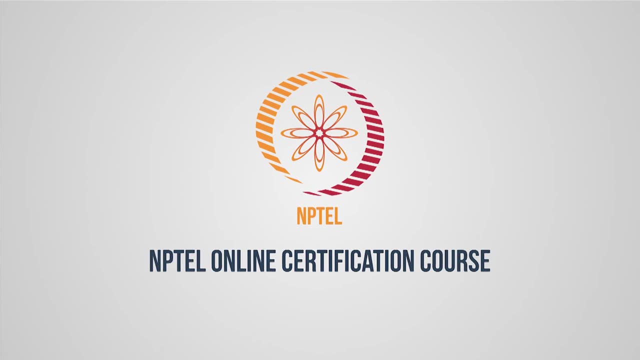 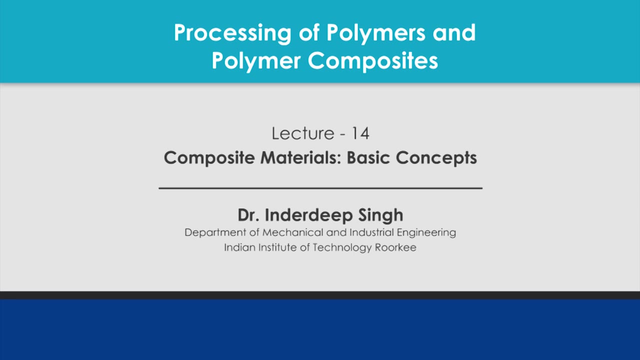 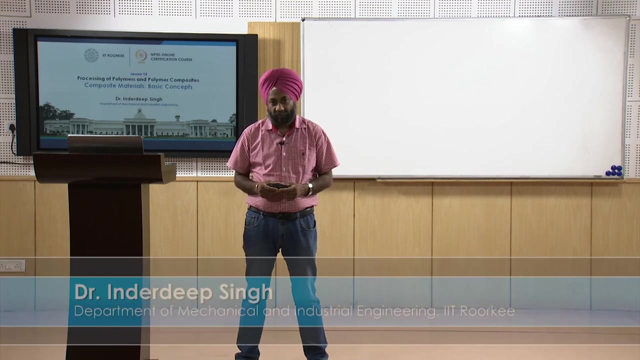 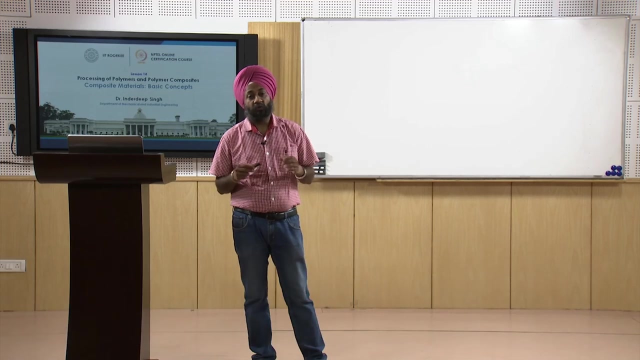 Namashkar friends. So we are done with our discussion on processing of polymers and we are going to start a completely different aspect of polymer based composites, or we are going to start our discussion on composite materials Now. the today's session will be: 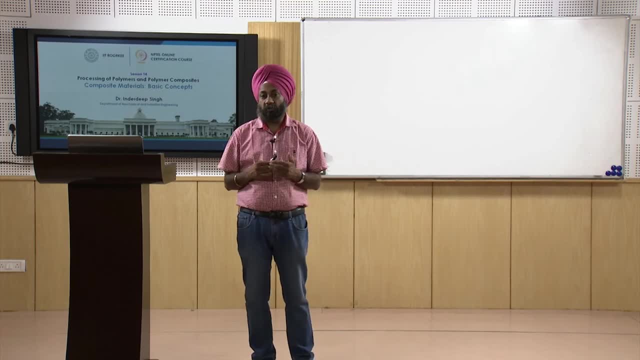 a kind of a fundamental lecture or fundamental discussion on the concept of composite materials. Now we have discussed polymers, So we, we can add, you can say that is a different types of polymers we see around us. they have different types of colors- red color polymer products. 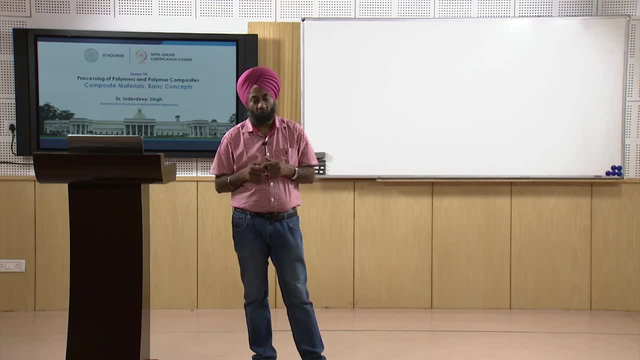 or plastic product. blue color plastic products, green color plastic products? yes, they do exist, but the basic color of the polymer which has been used to make that product may be different. So some coloring agents are added into these polymers, So can we call these? 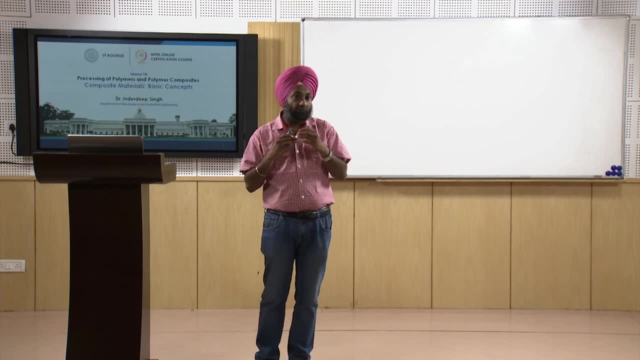 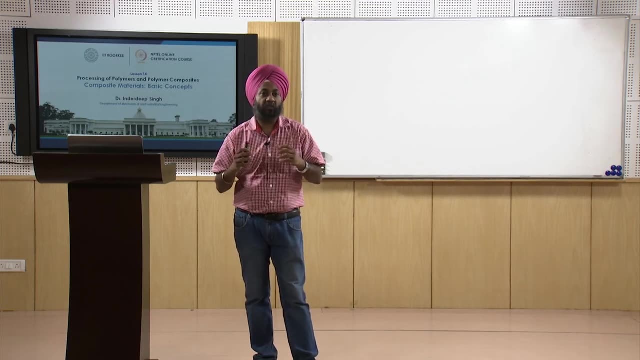 products as composite products? no. So we have to be very, very clear that which material we are going to call as the composite material, And that is the object of our discussion today: that we try to understand that. what is a composite materials? composite material? There is there a large number of lectures available on composite. 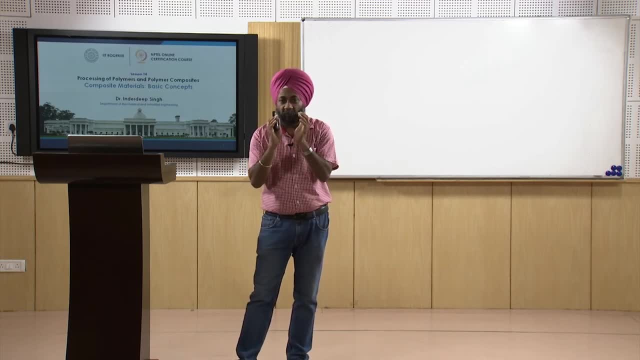 material. So we will just try to understand the bare minimum fundamental of a composite, and then our topic is processing of polymers and polymer based composites, or polymer composites. So our focus would be to discuss the processing routes, processing technologies or fabrication. 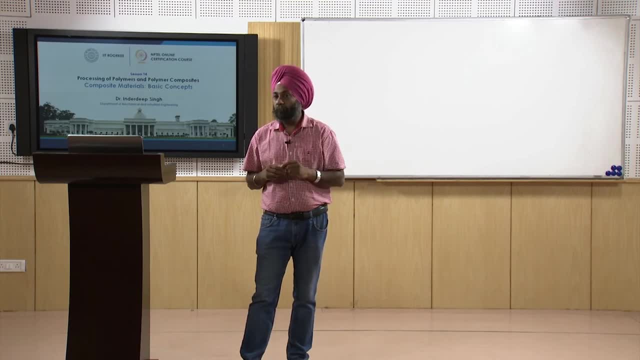 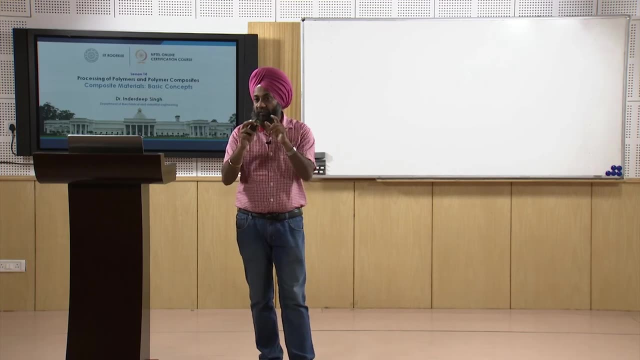 technologies for various types of composite products and specifically polymer based composite products. but as one word that is coming in our title, that is, processing of polymers and polymer composites- composite word, we should try to understand that what is basically a composite material? and if we can understand what is a composite, we can work in different. 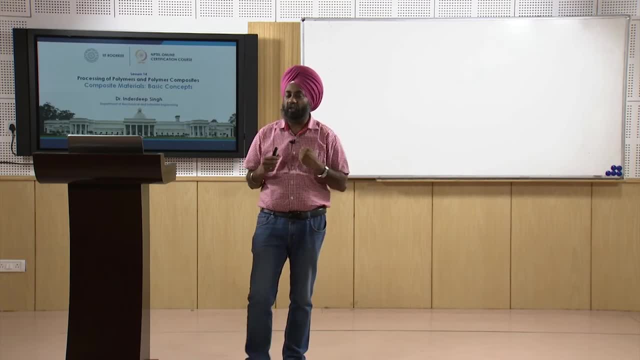 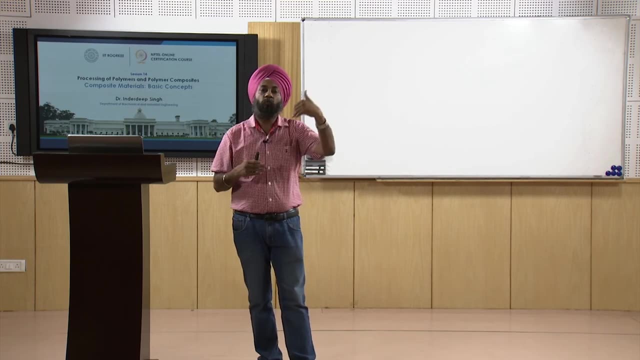 dimensions of composites, right from conceptualization that what can be a matrix and a reinforced reinforcement, to the fabrication, to the characterization, then finally into the application part of the composite. so first and foremost we should try to understand what a composite material is. there are number of naturally occurring composite materials. 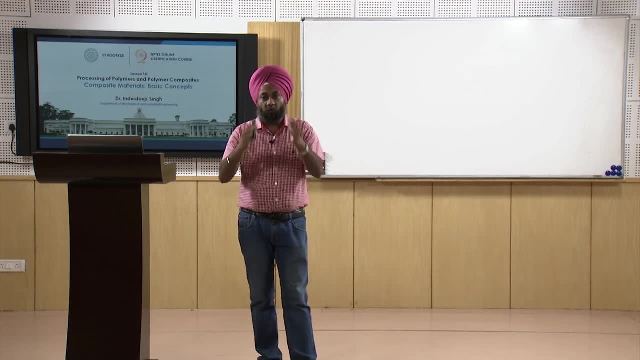 our forefathers used to make the mud walls in mud houses, so you. they used to mix the vegetable waste, the agricultural waste, the compost with the mud in the form of small fibers, and then they used to paste it around the mud wall. so what was the purpose of that? we need to understand it. and composites give. 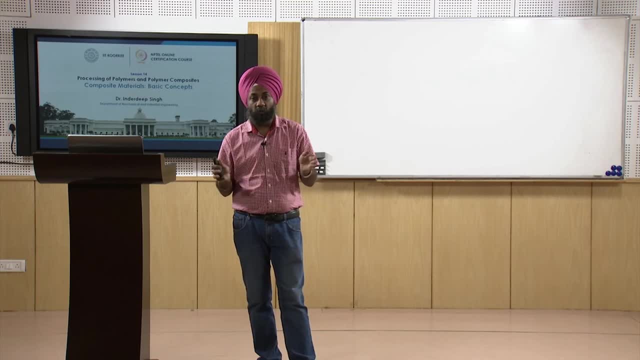 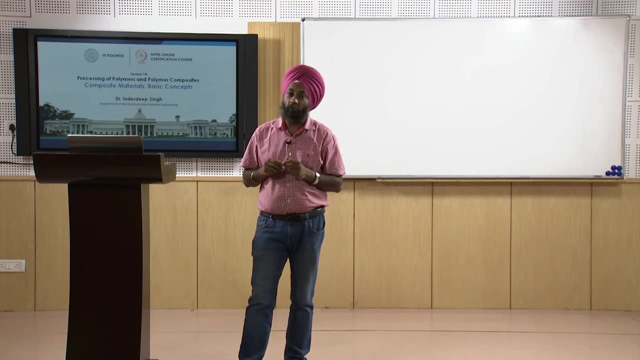 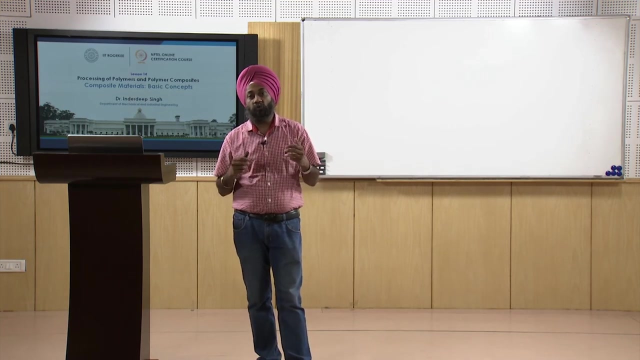 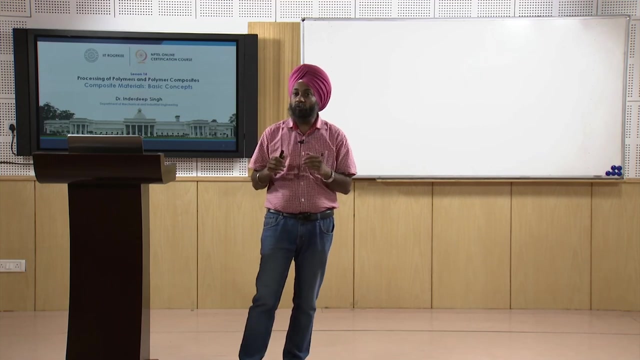 us the answer to this question, that why do they add all these agricultural waste into the mud? why, what was the purpose of that? so that is one fundamental query that we need to an answer. then our bones- human bones, animal bones- are also examples of naturally occurring composites. even wood is an example of naturally occurring composite, so i am not going to explain. 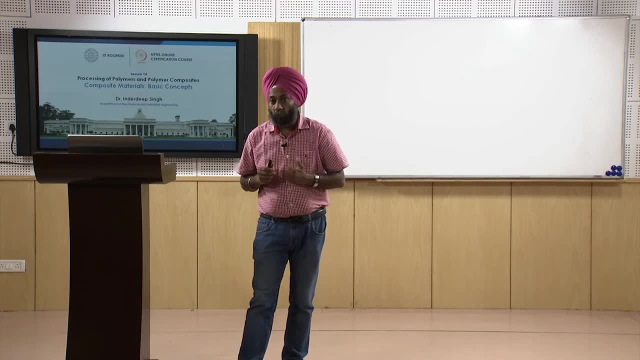 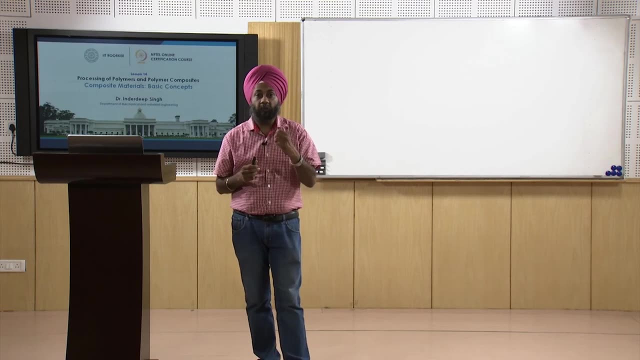 what are the constituents of wood or, ah, human bones. but you need to find out as an assignment that what are, what are, what is present in the wood, what can be termed as matrix in context of a wood, what can be termed as reinforcement in context of a wood? similarly, in bone, what 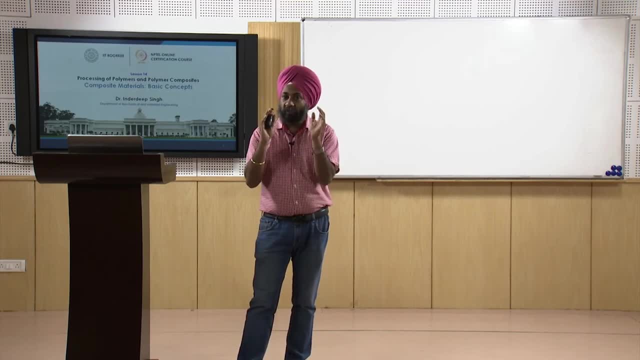 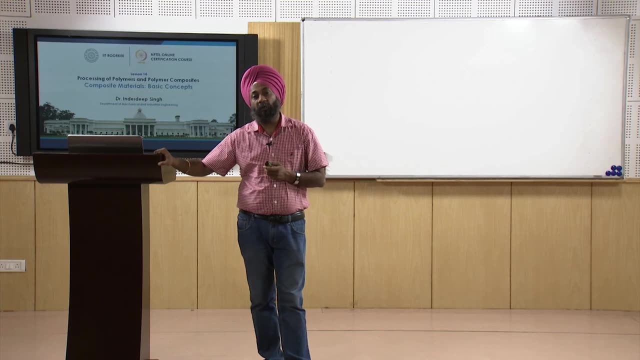 is matrix? what is a reinforcement? but what are the basic terminologies that are present in the wood? i say what is the basic terminology of a composite, so i am not going to explain. is related to matrix and reinforcement that we are trying to go cover today in the form. 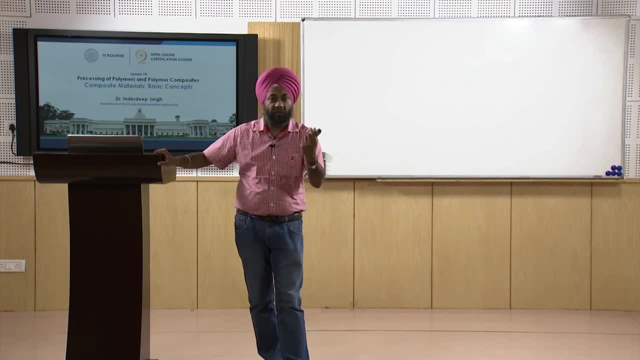 of our session and we will see that in a composite. what is a reinforcement, what is a matrix? so let us start our discussion with the composite material and first example that usually may not be that true civil engineers can give a better representation of that. ah, you can. 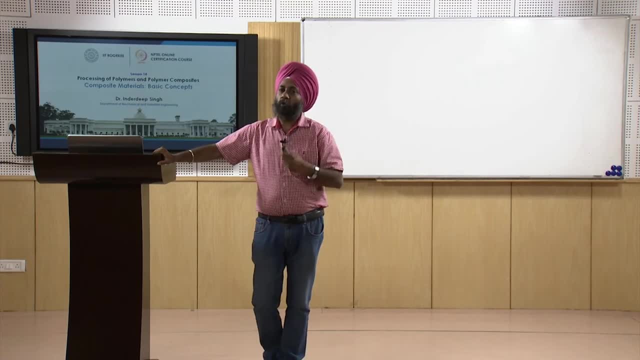 say analogy, but one example that i usually quote whenever we start our discussion on composite materials is the rcc structure. so we have concrete and the metallic rods. now the concrete. if you see all the time, it is made up of so many different mixture of so many different civil engineering materials. but cement is also one of the important parts. 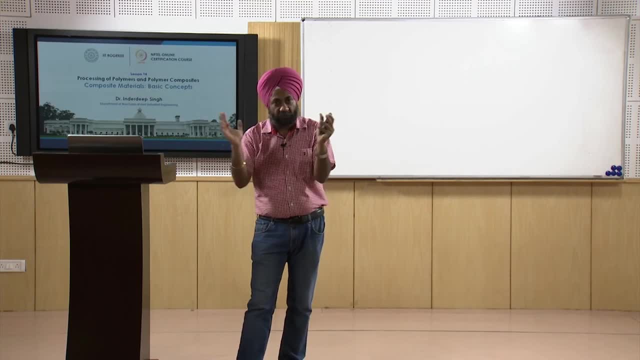 there and in cement, always we talk of the compression, always we talk of the compressive strength. we can say: concrete is good in compression but it is poor in tension, whereas the metallic rods are good in tension but are poor in compressions. if you ah apply a compressive load, the buckling 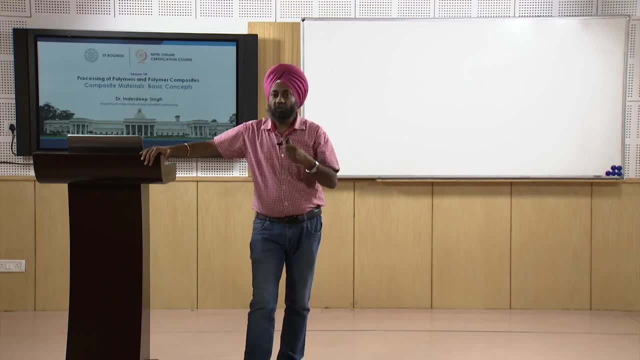 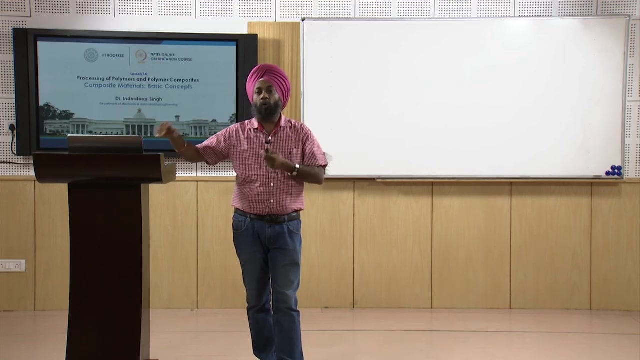 may take place. so what simple example just to can explain the concept of matrix and reinforcement. now we have combined concrete and the metallic rods together into a civil engineering structure. why? because we are want to take the advantage or the best of the virtual off duties. but this four parts specific material is called concrete, which 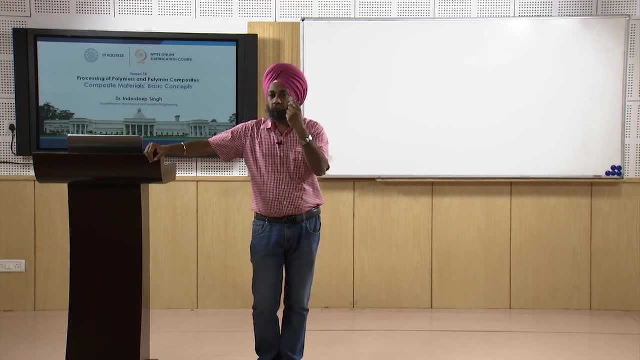 is corrival together. then you can have the другие concept. it is called compressed real materials, that is used in the spices, as well as metal rods, that is called environmentally, and BO is all about the running process. so all these three, the property of both the constituents, that is, the concrete, as well as the metallic rods. 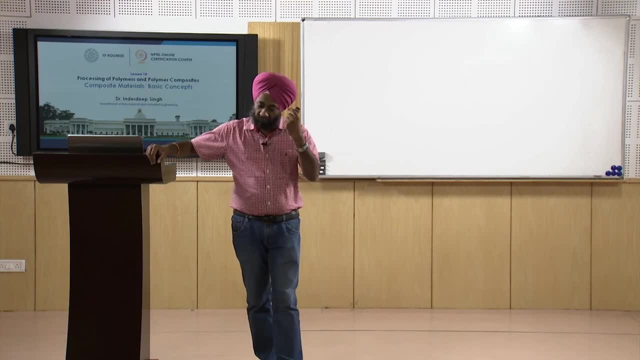 so from here, which derived the concept of ah, ah, reinforcement and a matrix. so in this case the continuous phase is concrete. so if you see, first we have a networks of the metallic rods and then we put concrete, so concrete you can see encapsulate all the roller. so 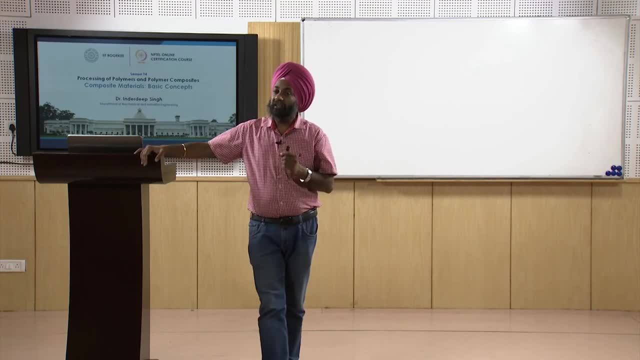 concrete is the continuous phase here and therefore we can say, showcasing the source of the material ball that is called concrete, core p? u, the concrete which will guest in the anytime concert of the metal, metal steel we put, get packing. Hari's also done any such say that concrete is the matrix in this case and the reinforcement is being provided by. 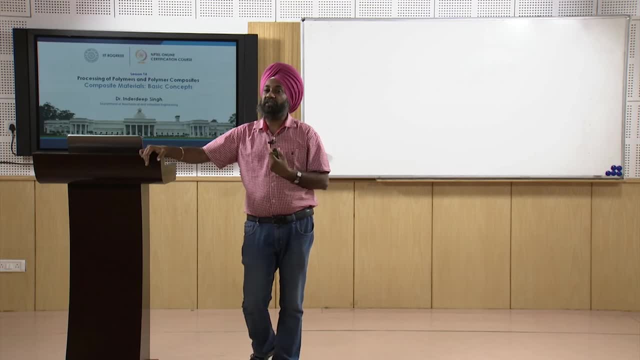 the metallic rods. so we say the metallic rods are acting as the reinforcement and concrete is acting as the matrix material. so for all types of composites we will see that it can broadly be the ah, categorized into two main constituents. one constituent will be a matrix, another constituent will be a reinforcement. and based on the matrix and the reinforcement, 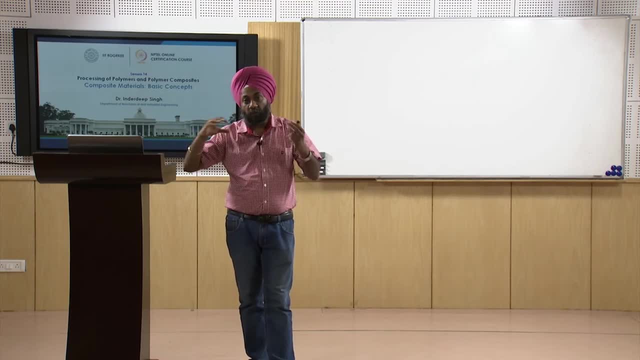 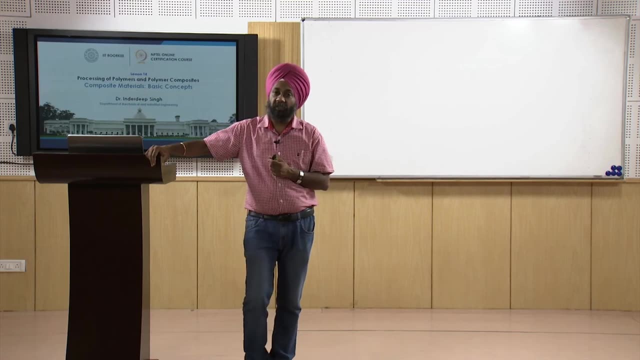 their chemical nature and further their physical form, further their properties, mechanical properties. we can have different types of composite materials, so we can have matrix which can be ceramic in nature. we can have a matrix which is metallic in nature as well, as in our case. we can have 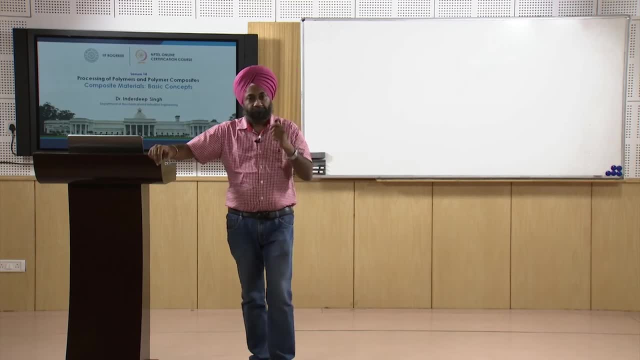 a matrix which is polymer in nature. so based on the matrix, we can have different types of composites. similarly, based on the reinforcement also, we will have different types of composites. now the reinforcement can be continuous, as in the case of rcc structure. it can be discontinuous or randomly oriented. 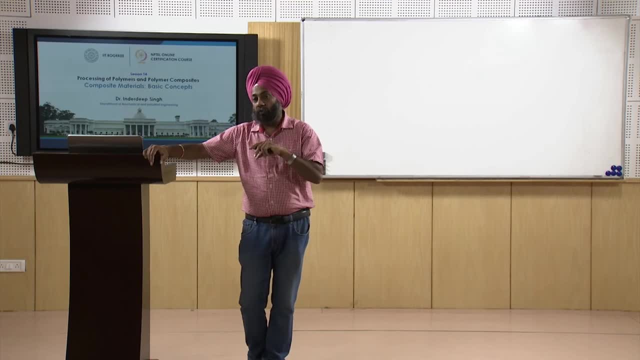 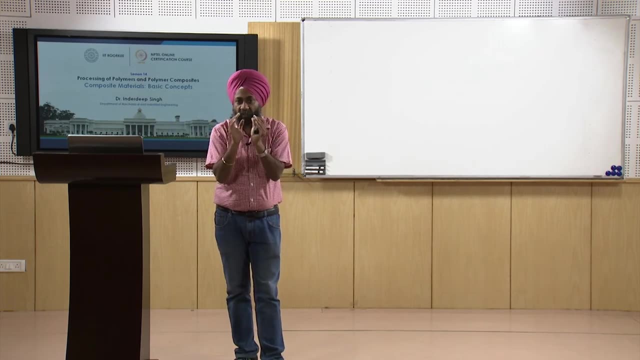 in case of metal matrix composite. so depending upon the types of reinforcement we can have different types of composite materials. so with this ah basic may be discussion. let us now switch over to our presentation and try to understand the basic structure in the case of a composite or in case of a metallic. 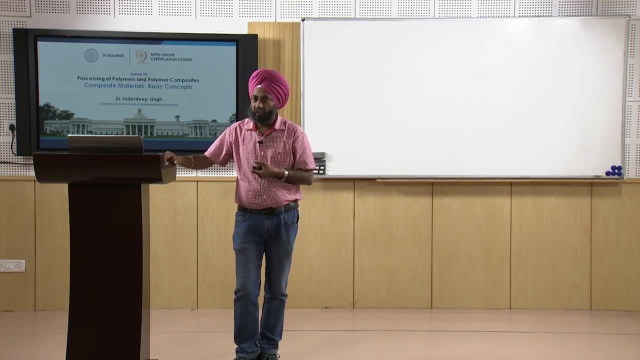 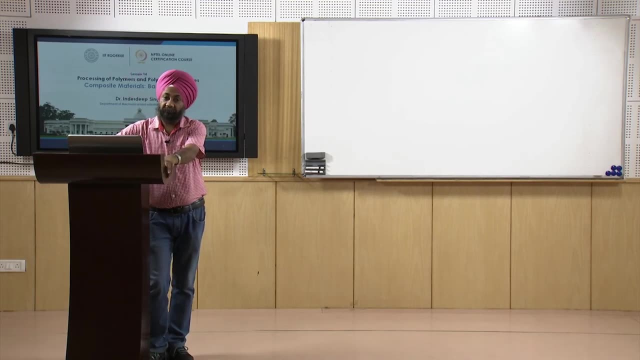 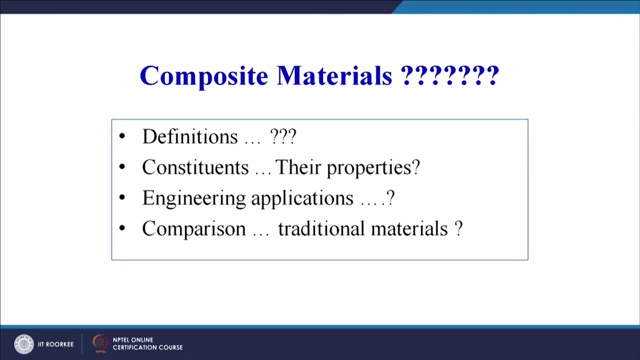 understand the basic concept, the basic definitions of the composite material. now, when we talk of composite material, we need to understand definitions, we need to understand the constituents. as i have told you, every composite material will have ah matrix, it will have a reinforcement. now, the properties of both, the properties of matrix, will be different. the properties, 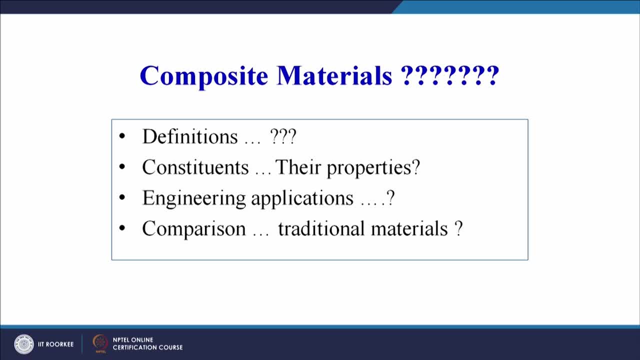 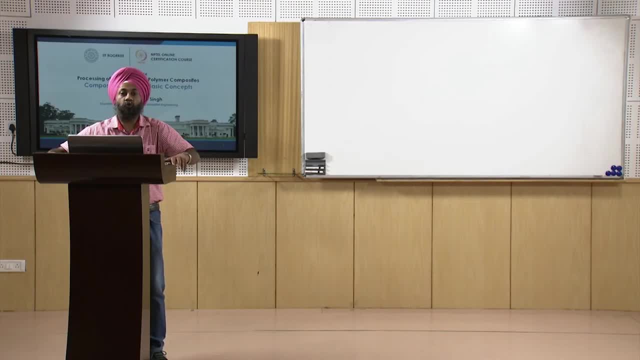 of reinforcement will be different now. we are combining two different materials with different properties and we are trying to make a single material. now the single material will have property distribution or a combination of properties derived from these two constituents. so we need to understand what are the constituents, what are their properties that are forcing 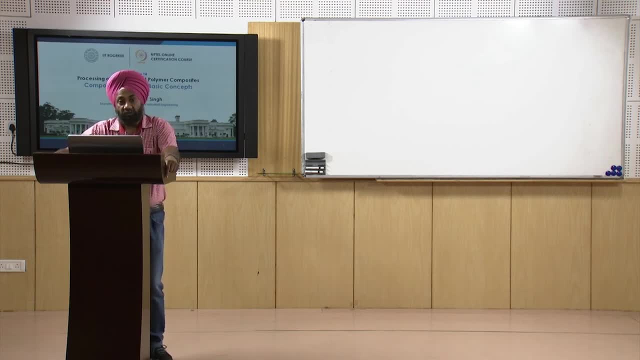 us to bring them together so that we need to understand, similarly, if we are developing a new material, what are the applications of the new material. if you are developing a new material, then what are the desire when you have to do these things? what do we need to do? so these parameters are going to help us to generate after, possibly. 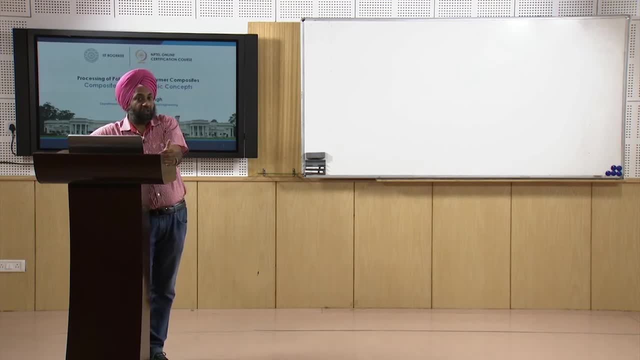 achieve these means we give a variable, a variation of that material and the right value to that material, and so on. and so i think that is what we have to understand: that we need to learn the relationships with the properties of materials okay than the existing materials. so we have traditional engineering materials like steel. we have traditional 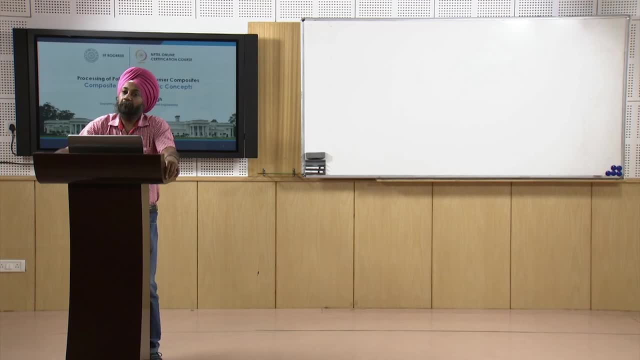 engineering materials like wood. so we have so many structural materials which are in use for maybe last hundred, fifty, two hundred years now. whenever you propose a new material, that material has to challenge and it has to overcome- we can say- the mindset. then it has to prove that it is a better material based on the properties, based on the performance. 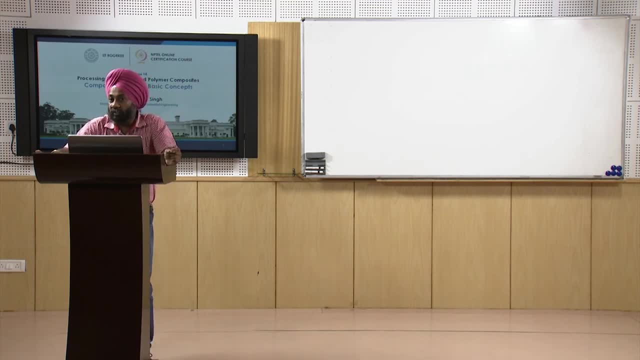 based on the in service performance. so that is also very, very important. that is, the comparison of ah properties of the new material as compared to the already existing traditional conventional engineering materials. so we have a whole list of conventional materials and composite materials. ah were developed in the maybe nineteen, sixties or seventies, so they are materials which are 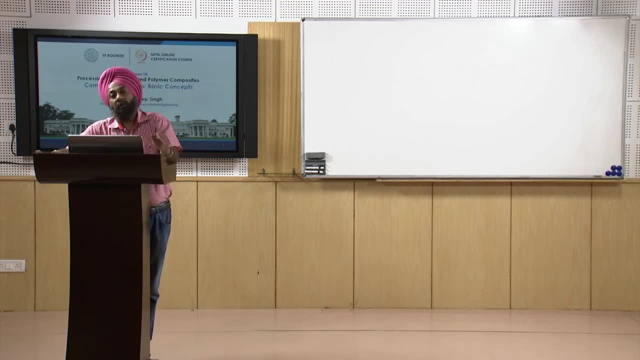 fifty, sixty years older, five or six decades old. so other materials are in, are in, may be. if you talk of the importance of materials, there are ages, historical ages, named after materials only. so the importance of materials is there since so many years. so whenever a new material is developed it has to overcome that challenge. 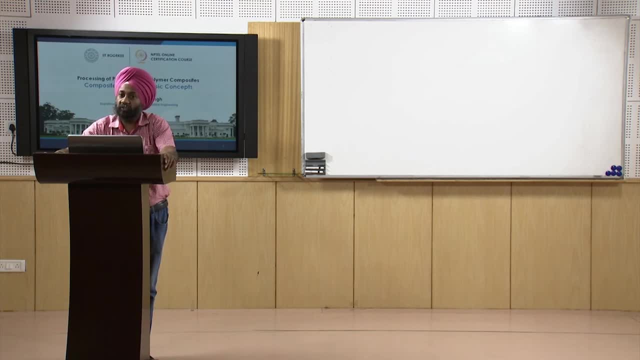 that? what is it going to achieve which cannot be achieved by the already existing material? so comparison always become very important part for the new materials, so the materials are important for the old, so different material materials are important in this. so they are very, very, very, very important. so when we end todays session, i think not all but answers. 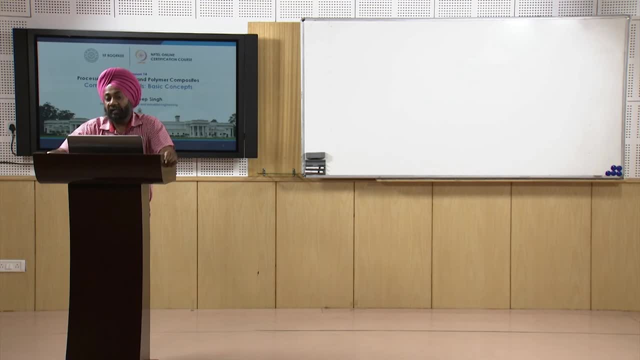 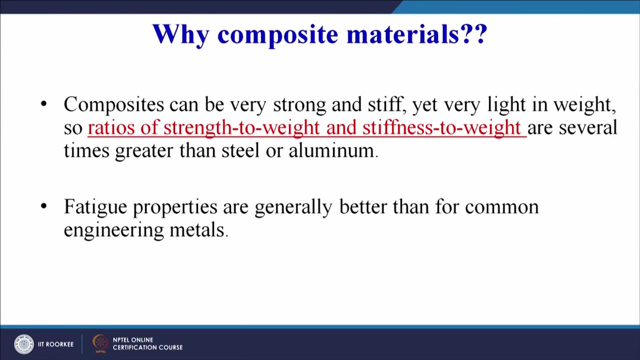 to some of the points raised or points highlighted in this slide should be clear in your thinking process. why composite materials now? first question now. composites can be very strong and stiff, yet very light in weight. so majorly, if we talk of the polymer based composites, 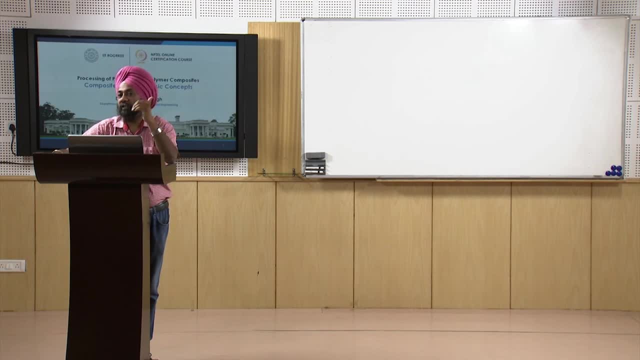 that is our topic. our topic is processing of polymers and polymer composites. so if we focus on polymer based composites, one of the major advantage is that they are light in weight. similar thing may not be true in case of metal matrix composites, but if we focus 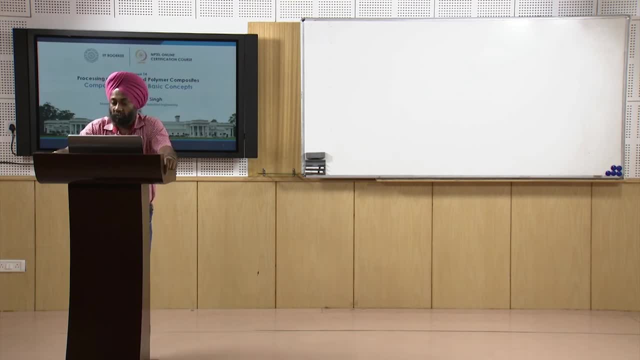 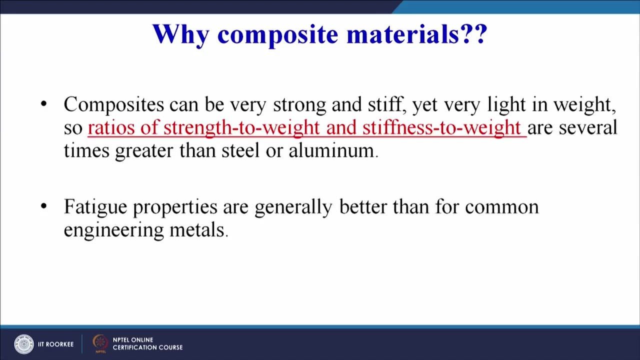 on polymer composites only. these are very strong and stiff and yet they are very light in weight. so the ratio of the composites is very important. so the ratio of the composites is very important. the ratio of strength to stiff, strength to weight, as well as stiffness to weight is very 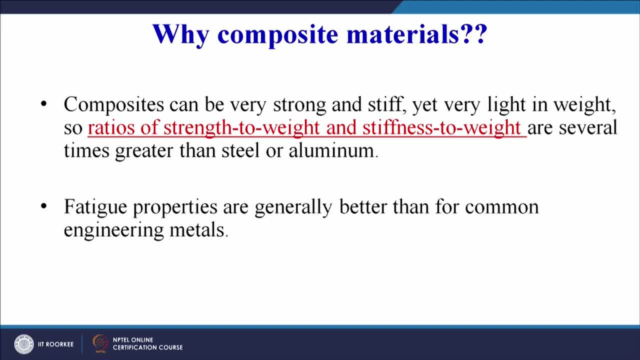 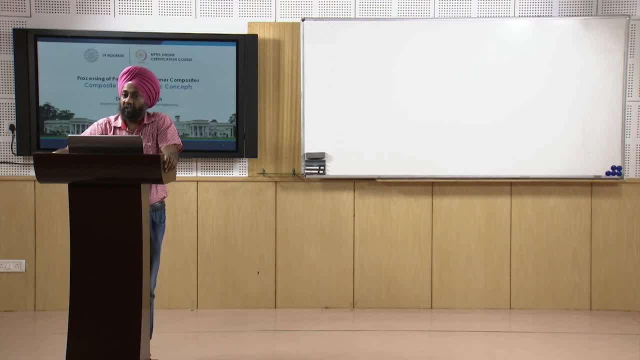 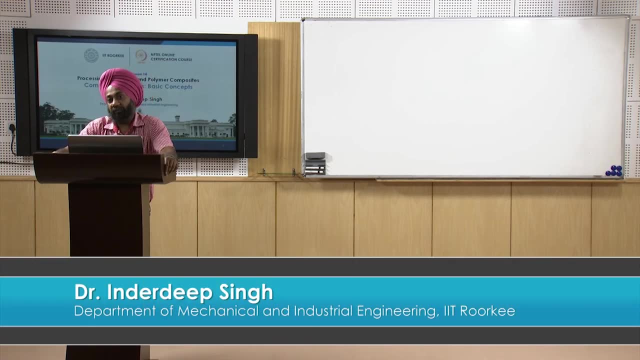 high and comparatively higher than steel or aluminium. so that is the point. in the last slide. i was highlighting that whenever a new material is proposed, it has to face the challenge of the traditional material. so for lightweight applications, we can conclude that these composite materials, specifically polymer based composite materials, have high strength to weight ratio. 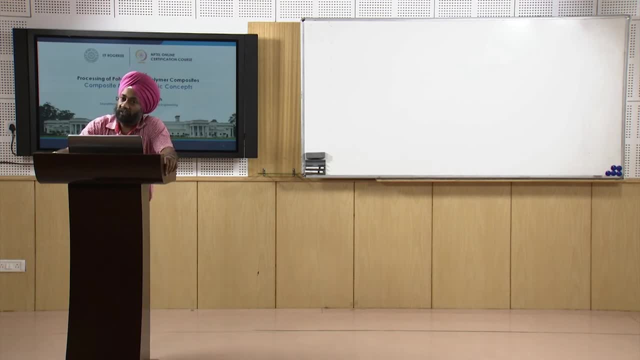 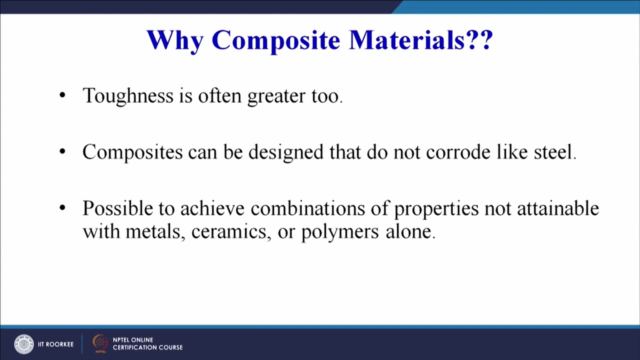 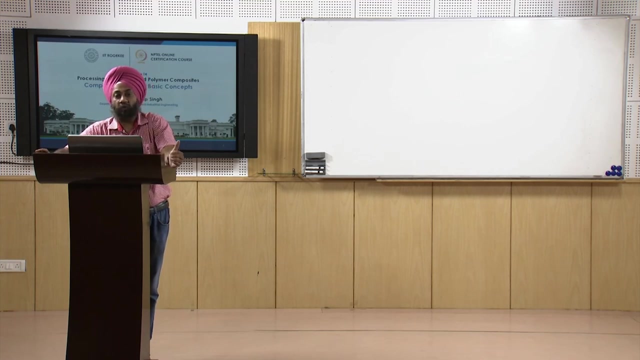 high stiffness to weight ratio as compared to the traditionally used metals, that is, steel and aluminium. moreover, the fatigue properties are also better than most common engineering metals. toughness is often greater too. so we can. we are comparing them from the mechanical engineering point of view. so we are talking. we are talking of strength to weight ratio, we are talking of stiffness to 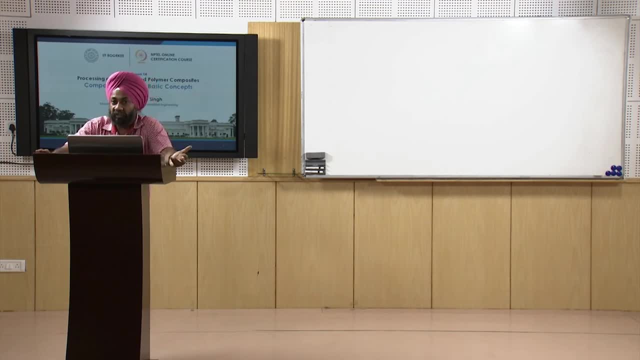 weight ratio, we are talking of fatigue, we are talking of toughness. now, all these properties are important from the applications point of view, so we can say that wherever we are using metals or wood, we can think of replacing these traditional materials with advanced materials, with materials which are light in weight. now, whatever discussions we have done, 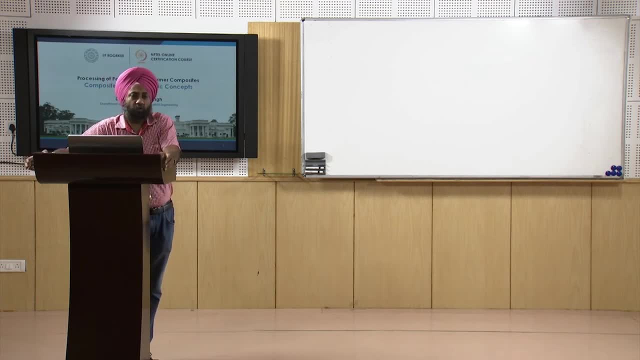 whatever discussion we have dealt in now, i may put a simple question to all of you: where do you feel that the maximum application of these materials can be? just give it a thought off. yeah, so the general question which we are thinking about. these materials are very similar. 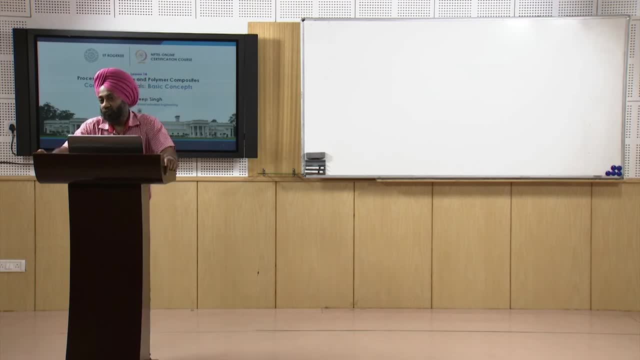 to medium weight applications or weight applications. so it is very simple one. we call them problem measures. i am not putting itjer reasons. you are also going to answer these. i would like to be really clear. my point is that, due to80 percent of time where these materials can, 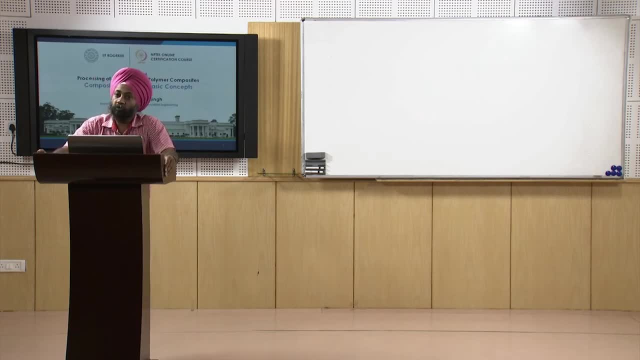 be used. now, if you can just look at uh properties, strength to weight ratio is high. stiffness to weight ratio is a lightweight application. so very easily you can see they can be used for aerospace industry. they can be used for making medical assistive devices like our crutches. so you can just 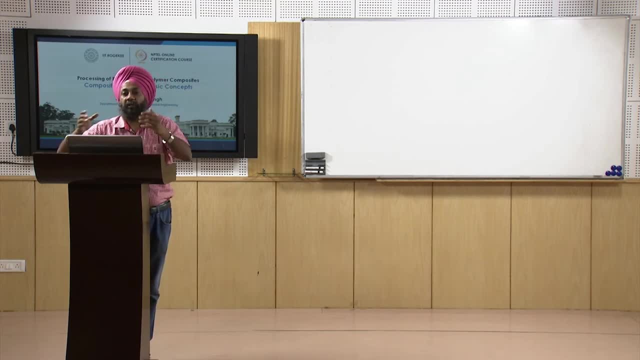 from light weight aspect only, you can find number of applications where these materials can find usage. so the mechanical properties. therefore, we are highlighting that these properties are comparable or many times better as compared to the traditional engineering materials. so therefore, in we can coming to slightly on the chemical side, composites can be designed. 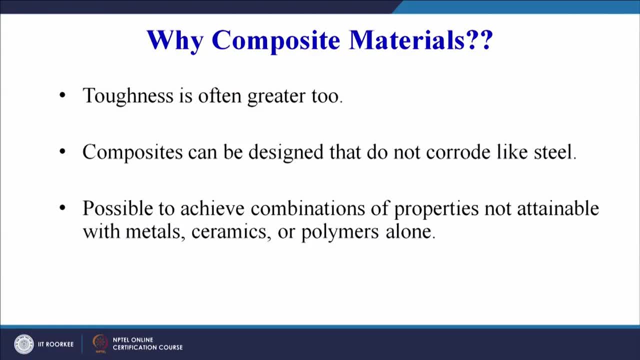 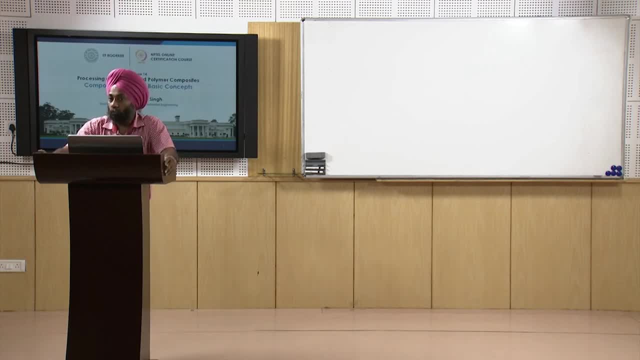 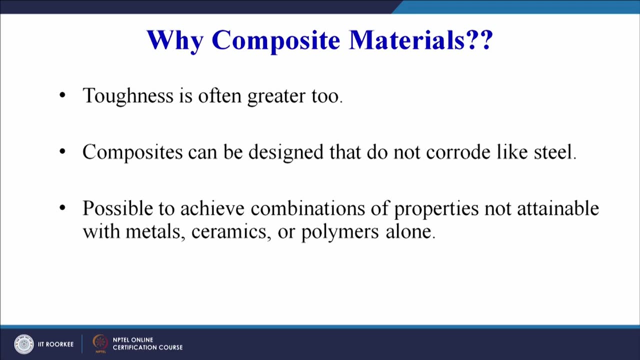 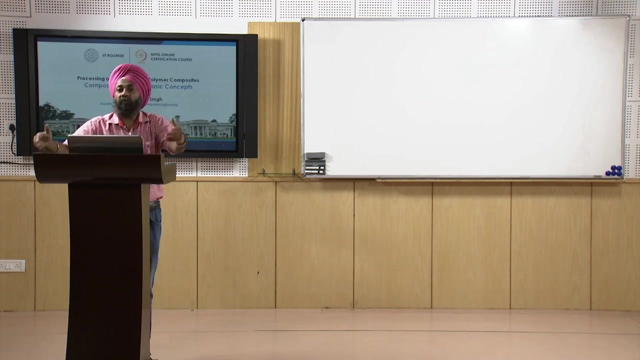 that do not corrode like steel. so mechanical properties are comparable or better. corrosion resistance they resistant. they can be made or they have the property of corrosion resistance possible to achieve combination of properties not attainable with metal, ceramics or polymers alone. now we can combine two or three materials together to make a composite material which 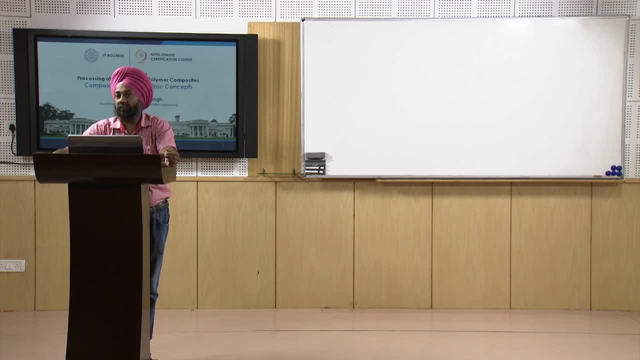 will have the same kind of materials, a very similar size, materials not attainable with metal, ceramics or polymers alone. now we can combine two or three materials together to have better properties as compared to the traditional metals, traditional polymers or traditional ceramics. now maybe the ceramics is the last word coming in our discussion. 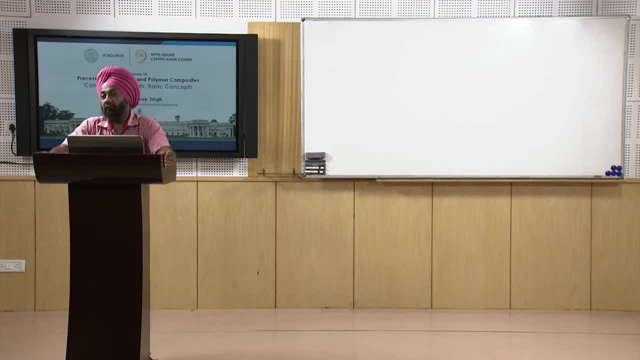 or ceramics, all of you know, has poor fracture toughness. now we can improve on that property by adding some fillers, adding some fibers into the ceramic, and it has been proved in research that addition of reinforcement in monolithic ceramics, or maybe pure ceramics, improves the fracture toughness property. so therefore we make the composite material. 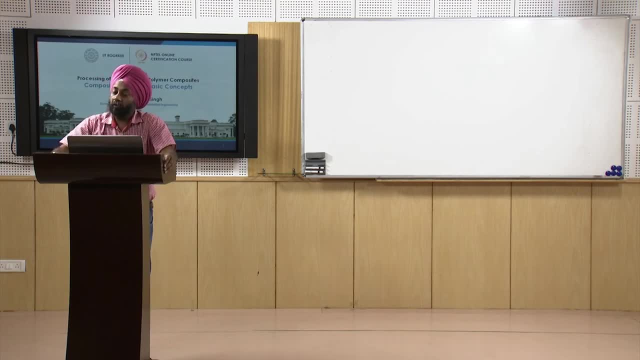 in order to develop a material, in order to conceptualize a material which will have better properties as compared to the constituents. now why composite materials? i think is very, very clear that we can attain the properties which are not available or not attainable by the constituents alone. so we combine the constituents together to make a third material. 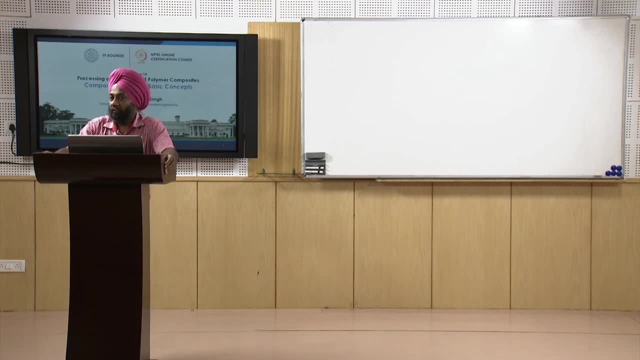 which has better properties or a combination of properties of the constituents. now coming on to the advantages. advantages are: they are tailor made properties. now, depending, tailor made means that we can design, we can make the measurements in such a way that fits the application. now, tailor made properties mean that these materials, we can select what is. going to be the matrix. we can select what is going to be the material that is suitable reinforcement. we can select the type of reinforcement, type of reinforcement, based on the shape, the size of the reinforcement, the form of the reinforcement, the quantity of the reinforcement. so as per the application, we can design our material. so that is first advantage of composites. 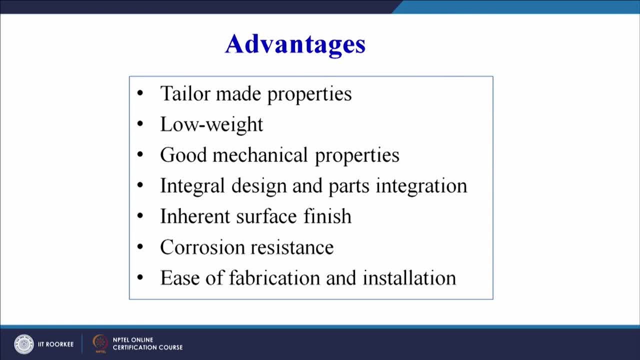 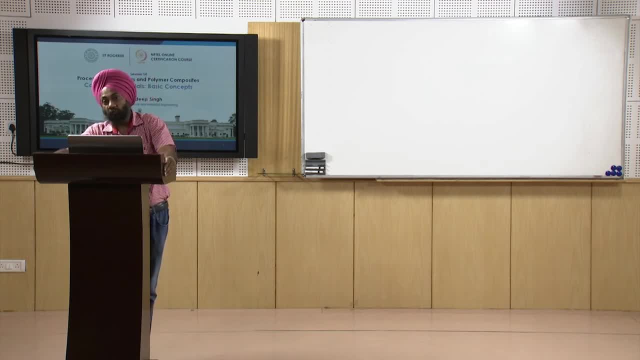 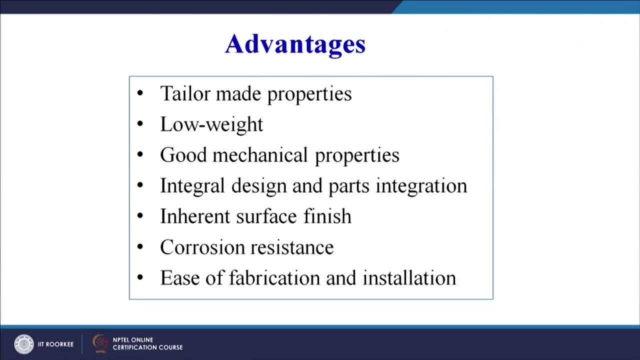 that they have got the tailor made properties. similarly low weight. already i think in our discussion today we have highlighted that they have high strength to weight ratio, high stiffness to weight ratio and therefore they are light in weight. good mechanical properties too. we have already touched toughness and fatigue. so they are, they have mechanical properties. 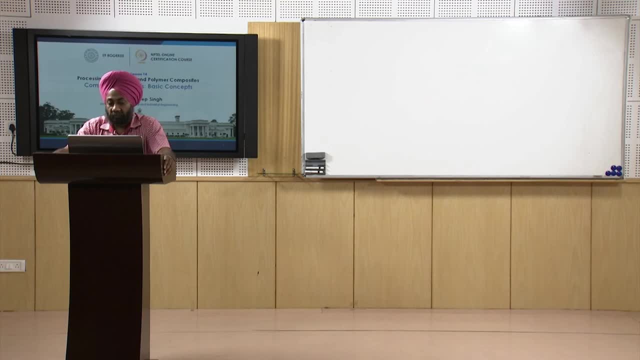 which are comparable or even better than the existing metals: integral design and parts integration. now, this is very, very important, because here the product is made in the form of dies or in the form of molds in. so they have got integral design, so we need not make two. 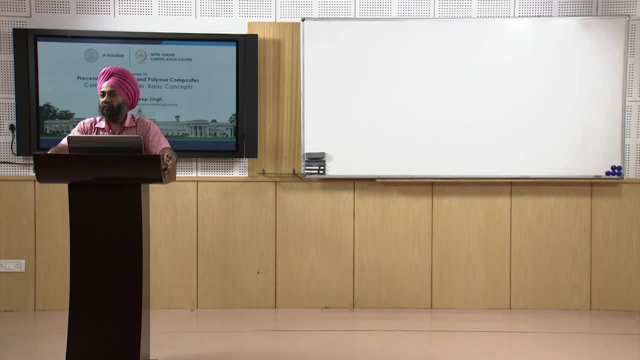 many different parts and then have problems of assembly. so here we can have a integral design and parts integration. so that is the second point, that we do need not make so many parts, so direct product can be made. we will see there are challenges in parts integration, also in case of composite material. but yes, that is one advantage and another advantage. 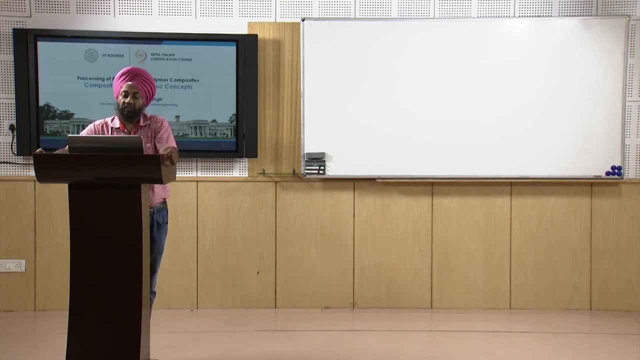 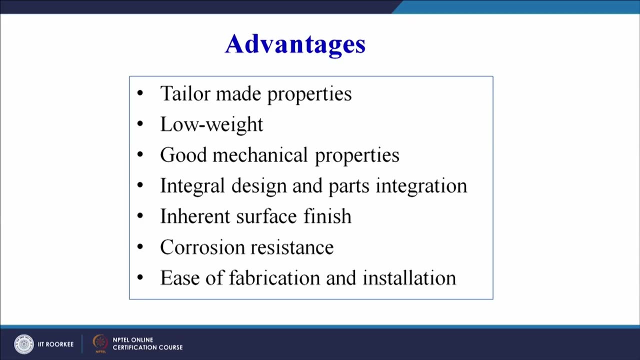 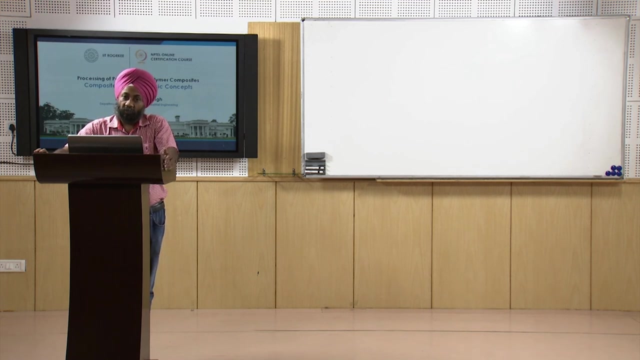 of the ah composite materials is the last point. i am, ah, just jumping two points. last point that is coming from integral design and parts integration, ease of fabrication and installation. now just take an example of a concrete bridge, or a traditional bridge that is made, or over bridge that has to be constructed. now it may take six months to. 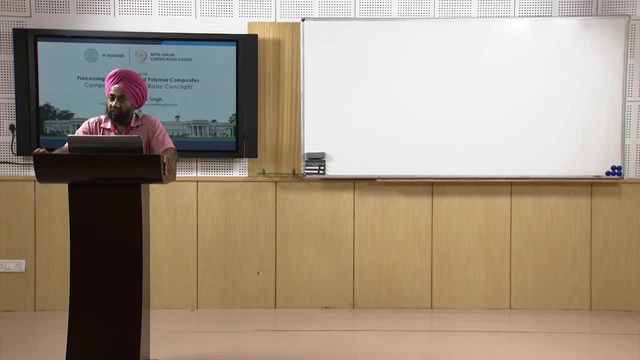 one year time to construct that bridge, whereas in case of a composite material, if you want to make the same bridge, same span length, all other dimensions or all other specifications remaining same, it will take may be a months or one and a half months time. why? because the composite slabs or the composite sections or the composite structural members will be fabricated in the industry or in the factory. they will be brought from the factory to the construction site and there only the final assembly will be done. so that is one advantage of with that is available with the composite materials, that it is easy to fabricate and easy to install. then other advantages are inherent surface finish. as i have already told you, composites will be made in molds and dies, so the surface finish of the dies will be replicated on the composite products and therefore we can attain or we can achieve very good surface finish as well as corrosion resistance. so i must address here that this list is not very exhaustive. 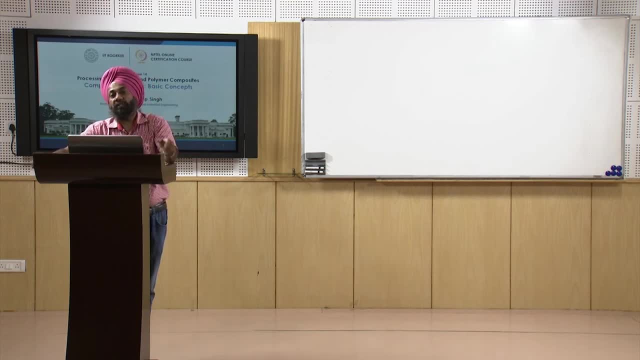 only six, seven points are given, whereas composites have got lot of applications and lot of advantages over the traditional materials. but yes, there are certain dark phases also. there are certain limitations also, for example, the flame retardancy or the frame retardant, behavior, inflammability, high temperature applications- this specifically polymer based composites are not very good. 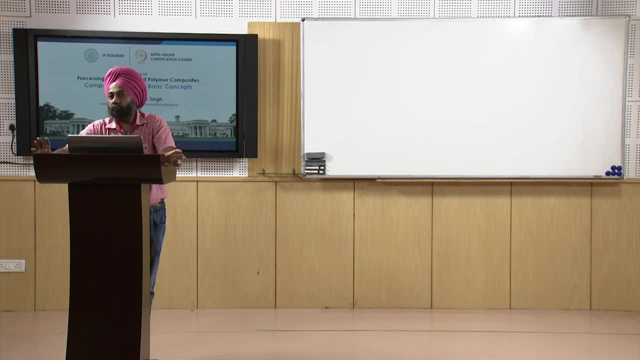 for high temperature applications. so there are problems also, but must i address that these are not the only advantages that composites possess. they have number of other advantages also which have been listed in different books and can the learners can address. those points may be on their own, but these are the major advantages that every engineer who has 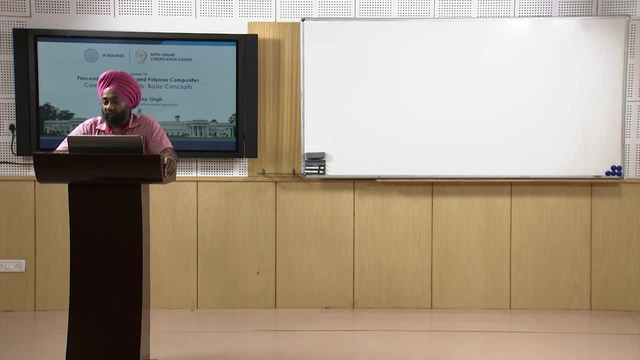 ah, fundamental knowledge of composite materials must know that. what are the major advantages of the composite materials? now coming on to the definition, the fundamentals. we have already seen that. why do we need to understand? why do we need to study composites and why do we need to study composites? and 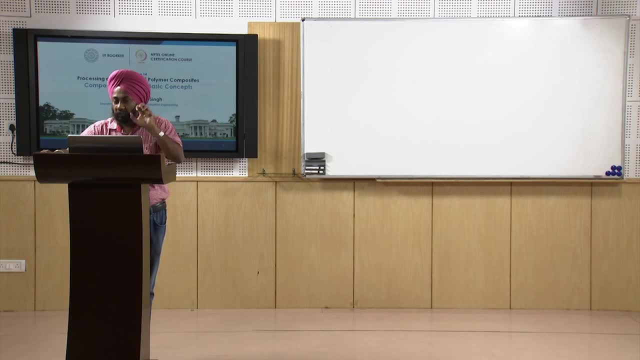 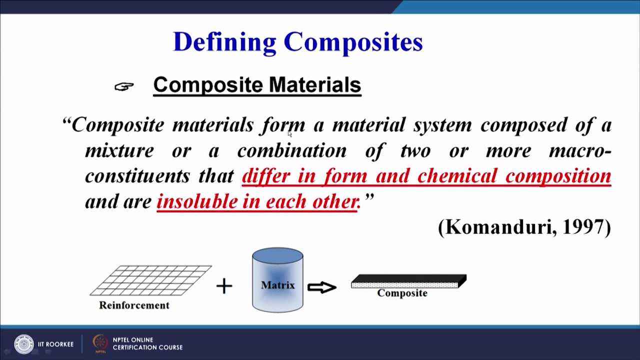 why do we need to study composing materials now? let us try to enter into the family, or enter into the basic concepts of composites. on your screen you have a very fundamental definition, given by common dury in nineteen ninety seven. composite materials form a material system composed of a mixture or a combination. 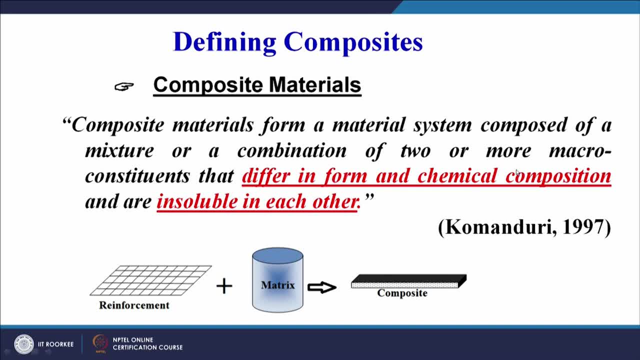 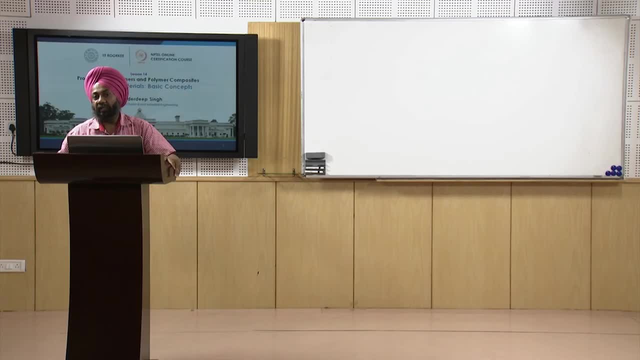 of two or more macro constituents. so that is one point. they are combination of two macro constituents. second point: that differ in form and chemical composition. now you can see that there will be macro constituents there. there can be two, they can be more than two, they can be three, they can be four. they 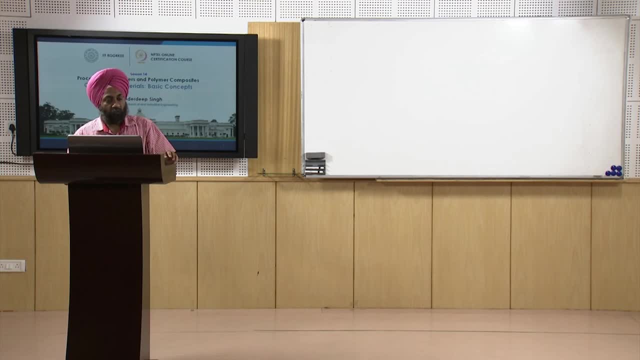 will differ in form and chemical composition. so maybe one can be, you can say, in the form of a polymer or a viscous fluid, other can be in the form of a powder, and then you are combining them so they are different in form. so one is viscous fluid, another one is powder. 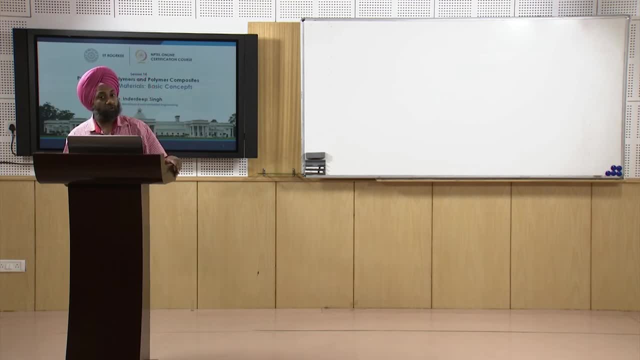 so that is a difference in the form, as well as the chemical composition is different and the last point that is most important, that they are insoluble in each other, and therefore i have given the example of rcc structure. if you break it, you will, you can separate. 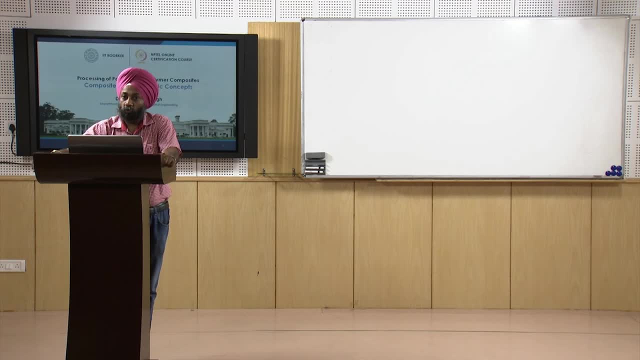 the concrete and you can separate your metallic rods. so the two constituents, that is, a matrix and the reinforcement, are not soluble into each other. they are insoluble into each other means they will retain their individual identity even after composite has been formed and there will be a interface. 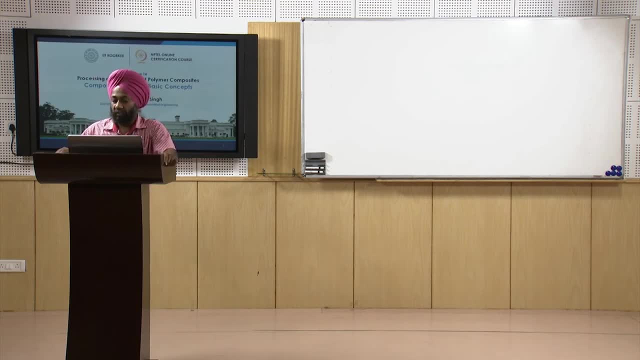 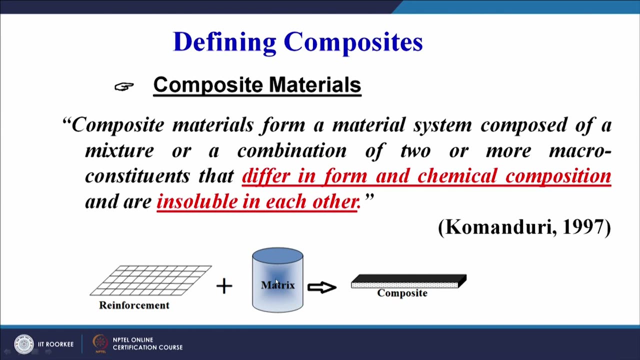 that separates the two constituents, that is, the matrix and the reinforcement. the figure is shown here. there is a reinforcement, there is a matrix, in our case polymer composites. polymer is the matrix material and they combine together. that is edition sign is shown here. they combine together to make a composite material. 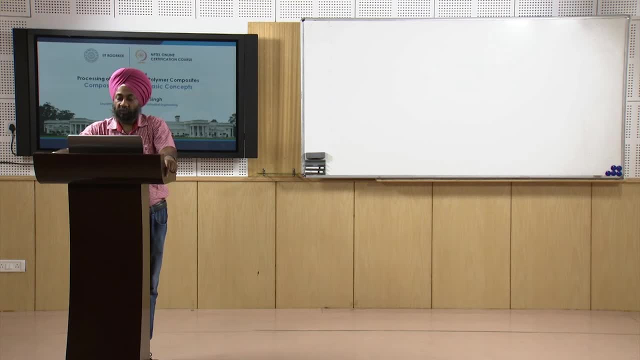 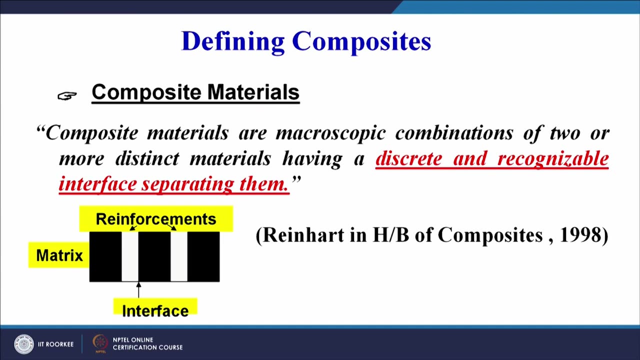 another definition. definition reinhardt handbook of composite. composite materials are macroscopic combination of two or more distinct materials having a discrete and recognizable interface separating them. so again you can see that there are again macroscopic combination of two or more materials. so there can be other two, more than two, three, four materials and they have a discrete and 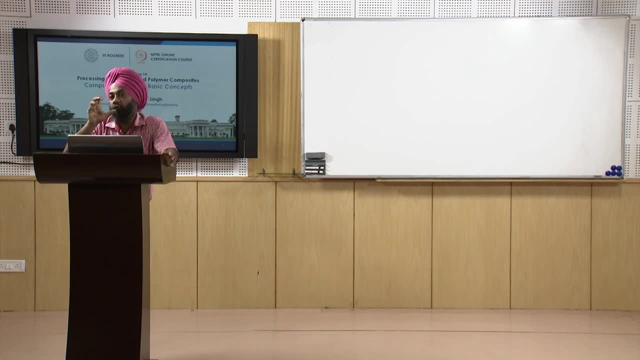 recognizable. so if you see under scanning electron microscope you must be able to see at high resolutions that this is the reinforcement, this is the matrix, and in between there is a interface that separates the matrix and the reinforcement. so on your screen we have shown a exaggerated view. the interface will not be this much thick in any composite, but 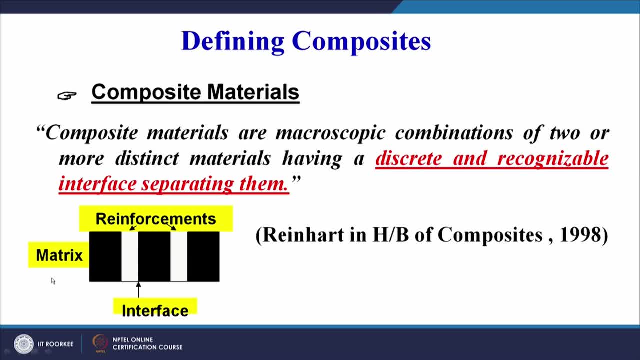 just to explain, we can see there will be a reinforcement. so there is a matrix. may be the black color is the matrix and the white color is the reinforcement, and there is a interface between the black and the white. there will be a interface running along this line and there will be a interface running. 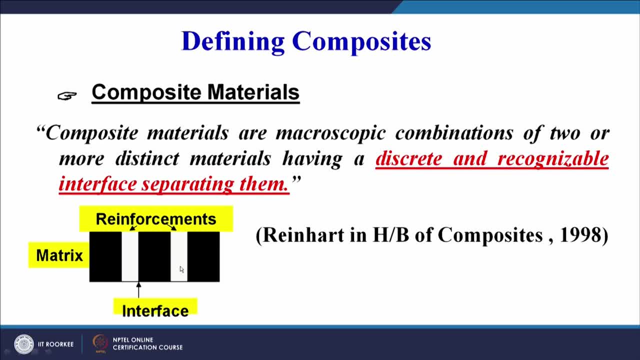 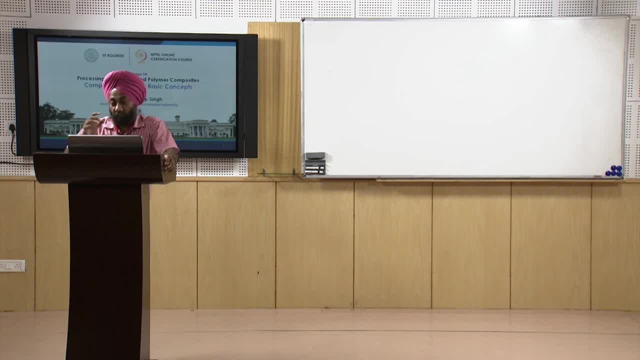 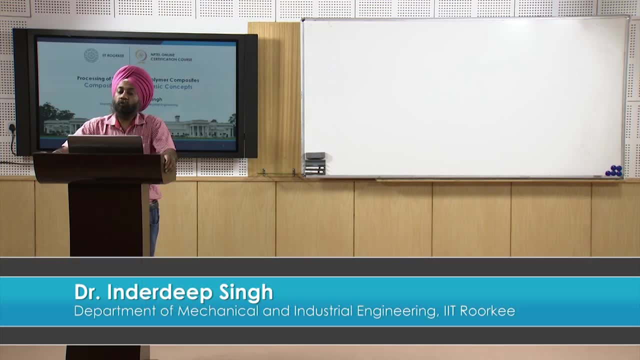 along this line. so there will be a interface that separates the matrix and the reinforcement. now let us try to understand the fundamentals of matrix and reinforcement. the components are constituents of a composite material. what is the matrix? what is the role of the matrix? matrix that holds the reinforcements. 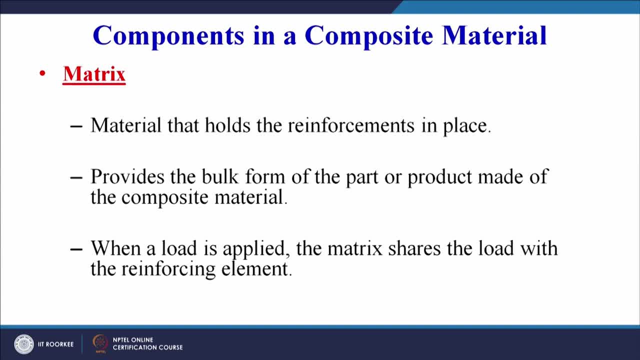 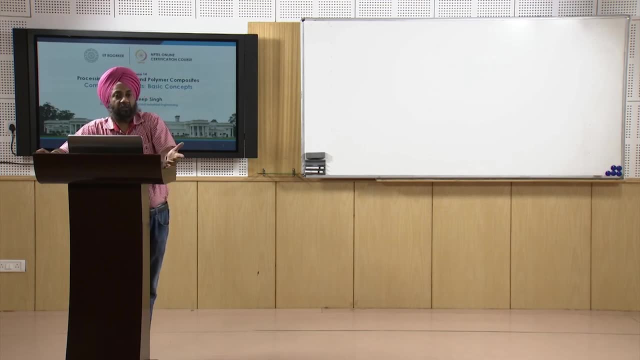 in place so it will keep the reinforcing materials to rather, or reinforcing agents together provides the bulk form of the part or product. we heard of the composite material so many times. you may have seventy percent matrix materials, thirty percent reinforcement reinforcement. eighty percent matrix material, twenty percent reinforcement, so the matrix forms the bulk. 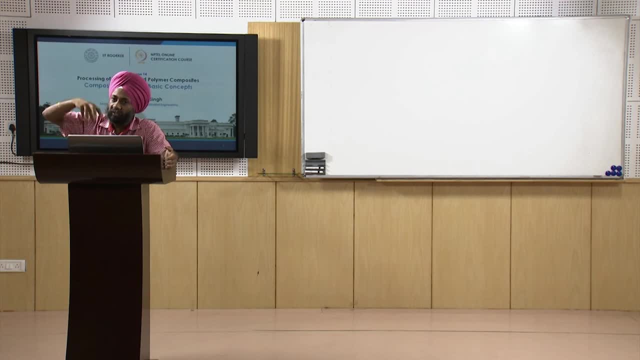 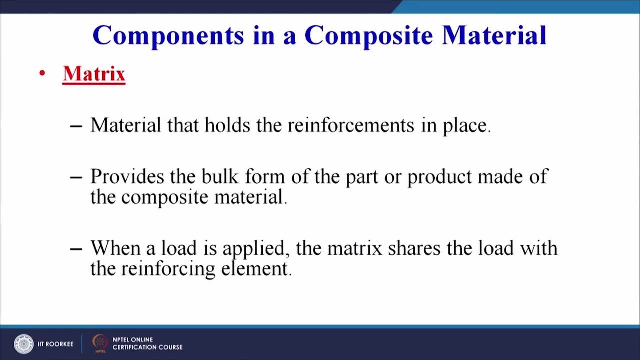 of the material. it is a continuous phase of its Hani soy and we reinforce it by putting some reinforcement. so matrix is the bulk or the main constituents, we can say, of the composite material. when a load is applied, the matrix shares the load with the reinforcing element. so in more technical terms we can say that matrix acts as a agent. 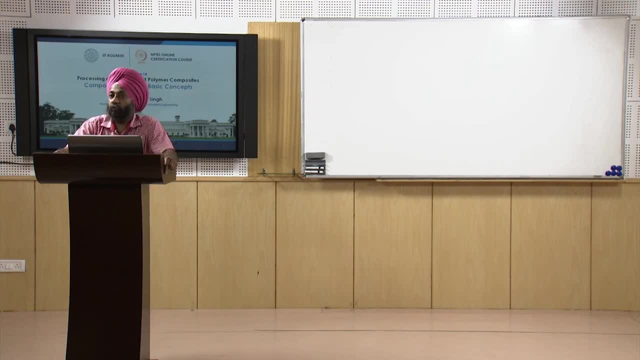 for distribution of load among the fibers that are used for reinforcing the structural member. so matrix acts as a agent for transfer of load. that is also one of the key objectives of the matrix. so majorly we will have three types of matrices. one is a polymer, as in our 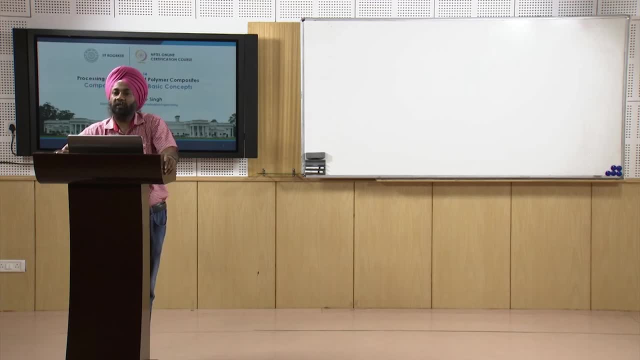 case, then it can be ceramic matrix, it can be a metallic matrix. so, for example, in metal matrix composite, we have aluminium alloy as a metallic matrix and it can be reinforced with certain ceramics such as a? l, two or three, or boron carbide. so, depending upon the combination, depending upon the application, depending upon 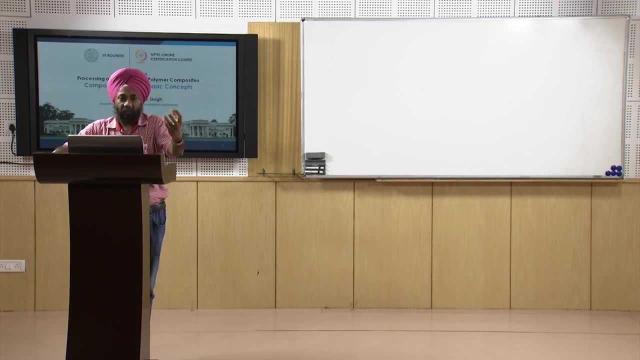 the desired properties. we may choose the metallic material as a matrix and we can use another, may be metal or it can be a ceramic as the reinforcing agent. so matrix based on matrix. we can have three types of composites: polymer matrix composite, ceramic matrix composites and metal matrix composites. 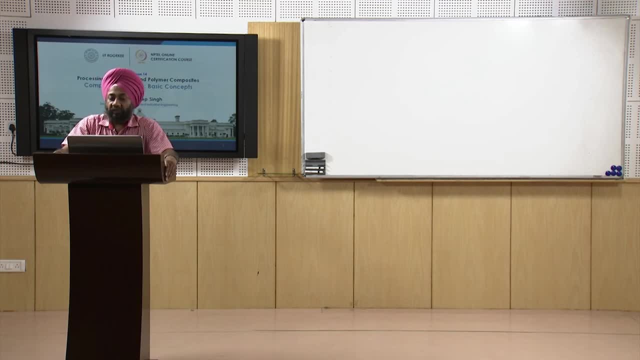 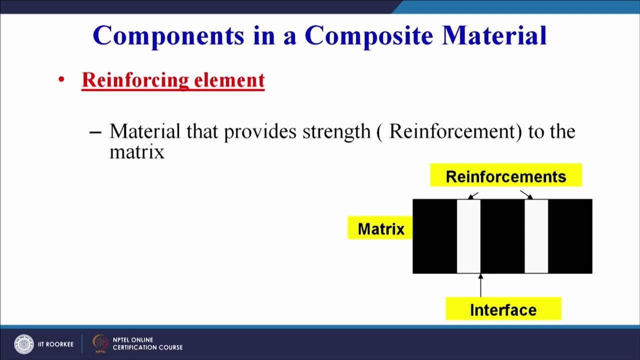 now the reinforcing element material that provide strength or reinforcement to the matrix. so we have this again. the same diagram is shown here. the white color portion is showing the reinforcing- or it can be reinforcing- fibers. the black portion is showing the matrix and there is a interface between the black and the white portion, which is, ah, separating the 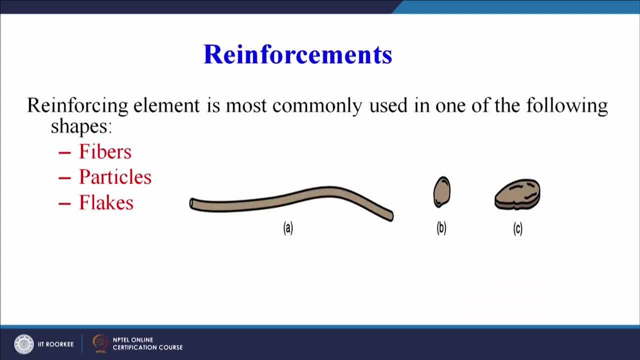 matrix and the reinforcement. now we can have different types of reinforcements. now reinforcing element is most commonly used is one of the following shapes. so maybe on your screen you can see different types of reinforcements can be used. so it can be fibers, it can be particles, it can flakes, it can be layers, it can be whiskers. so different types of reinforcements. 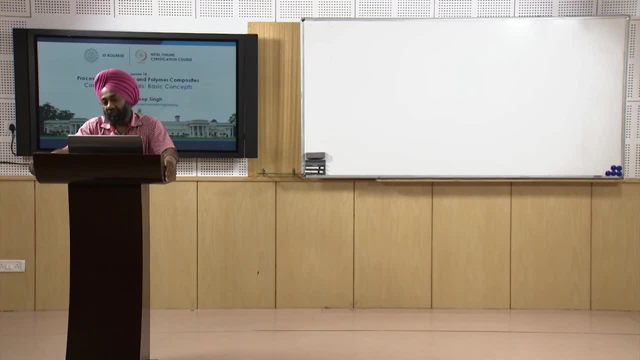 can be used for reinforcing the matrices. now, if the reinforcement concept is clear, the matrix concept is clear. now consider a and vector form here, and these are decided by the vu: Boni dagegen, Legend, saúde and behavior, earlier brain technology. We have the actual matrix concept for. 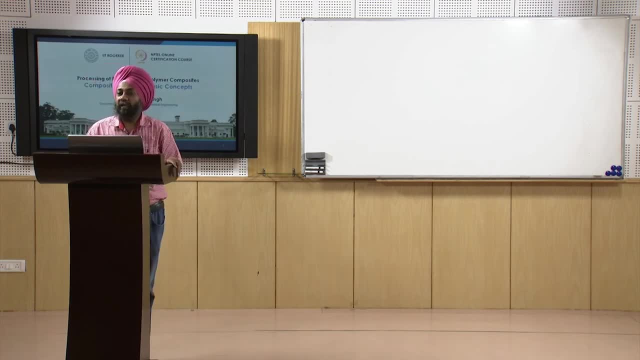 now, clearly, we can have a definition which will help us to differentiate the composite material from a alloy. it can help us to differentiate the material from a blend. so let us see that- how a material can be classified as a composite. now we can see both constituents are present. 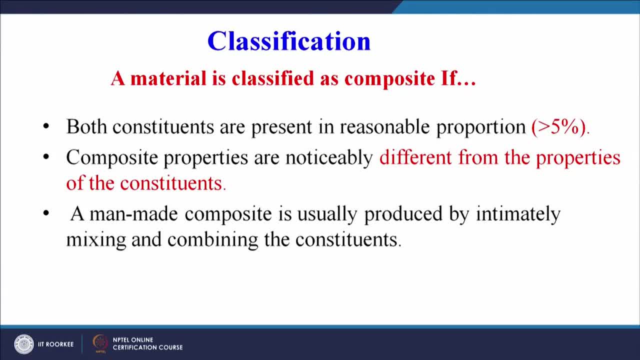 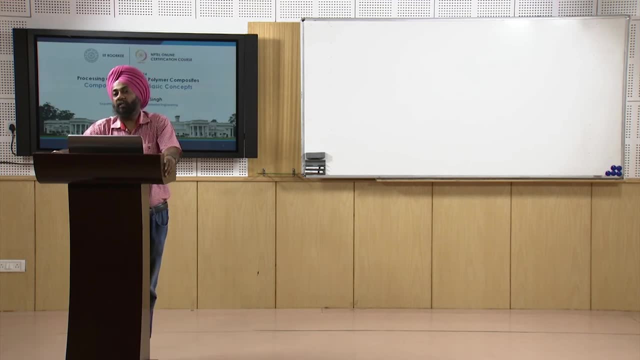 in reasonable proportion. that is the matrix and the reinforcement. for example, in rcc structure we can say the metallic rods as well as the concrete. both of them should be present in the rcc structure in appreciable amount or in significant amount and the bottom line ruffle rough. you can say: ah, rule of thumb is given that five percent is the minimum. 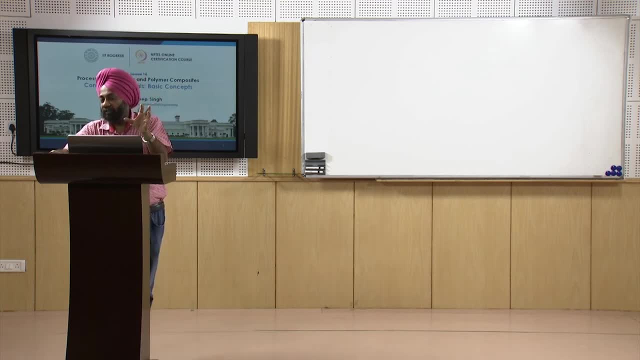 so maybe it can be a combination that matrix is ninety five percent and reinforcement is five percent. so we can say: ok, we can classify it as a composite material or a better. composite can be ten percent reinforcement by weight or by volume and ninety percent matrix, or it can be sixty percent matrix, forty percent reinforcement. so we can say that is one condition. 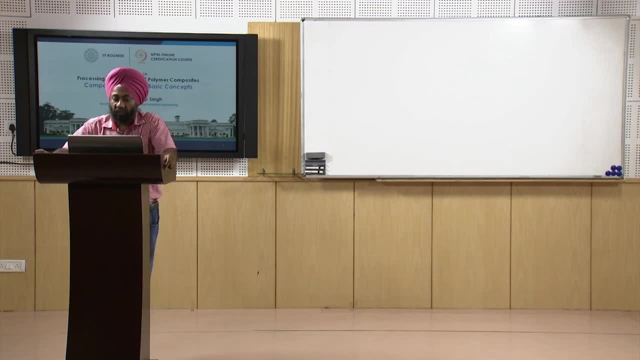 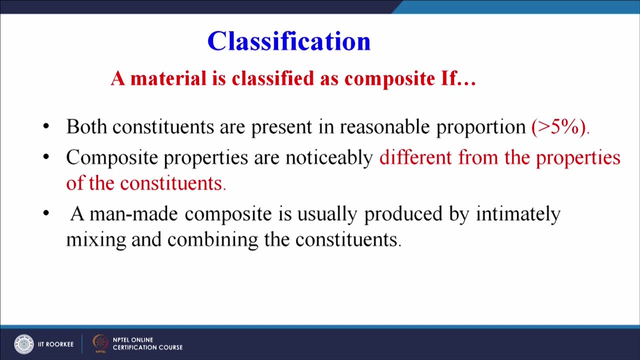 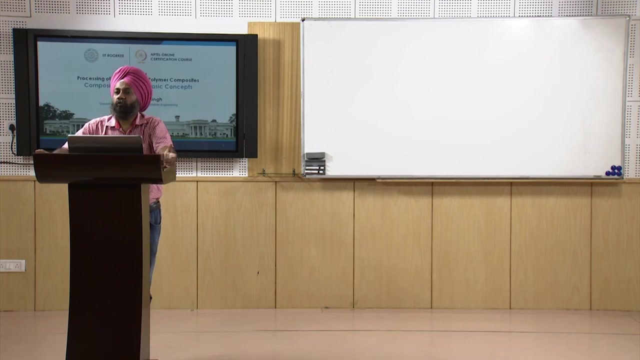 that both should be present in appreciable amount, then composite properties are noticeably different from the properties of the constituent. if one of the constituent maybe suppose the matrix is dictating all the properties of the composite, so we may say that what is the need of adding the reinforcement into the composite material? 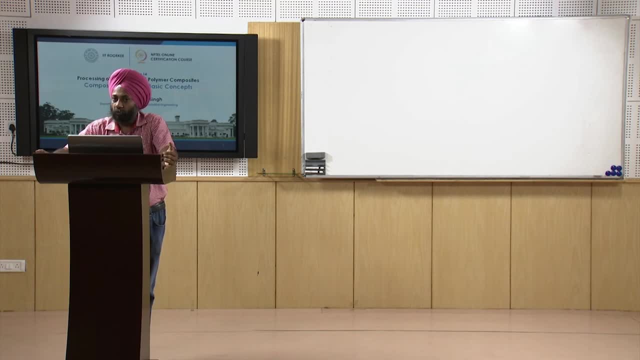 when all the properties are being dictated by the matrix only or, on the contrary, all the properties are dictated by the reinforcement. the matrix has no contribution in the properties of the resulting composite. then we may say that what is the role of the matrix? only reinforcement is maybe playing a most important role in dictating the property. so that is why we can. 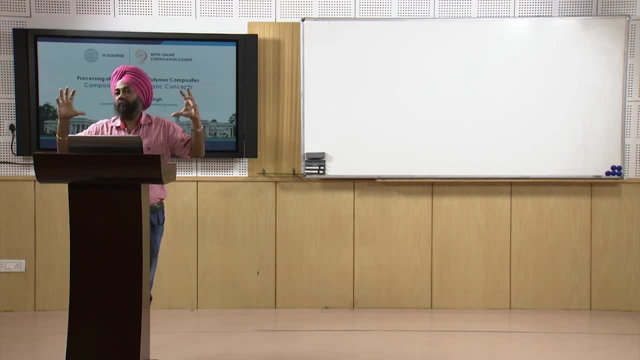 say, it is one important point that when we are combining two different materials together, we want to take advantage of the properties of both the material so that the third material or the composite that we are developing must have the properties or the better properties as compared to the two constituents. all the properties may not increase, but maximum property. 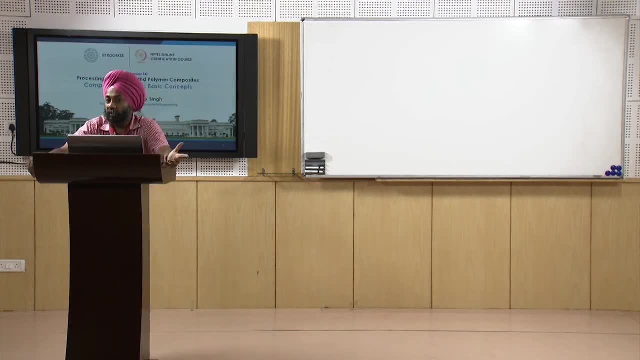 should improve by this combination. otherwise there is no need of combining the two different constituents, which are physically different, which are chemically different, which are chemically different. what is the purpose of combining them together if we are not getting desirable properties? The second point is the properties of the constituents should be different from the 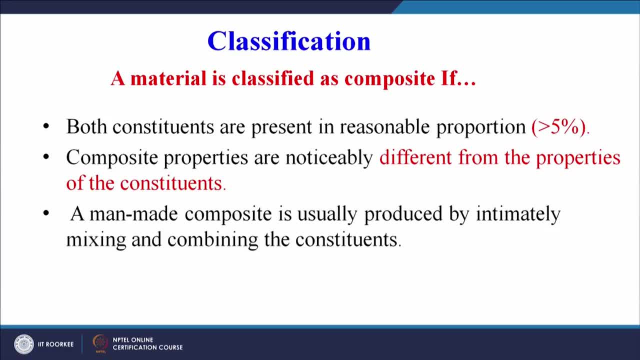 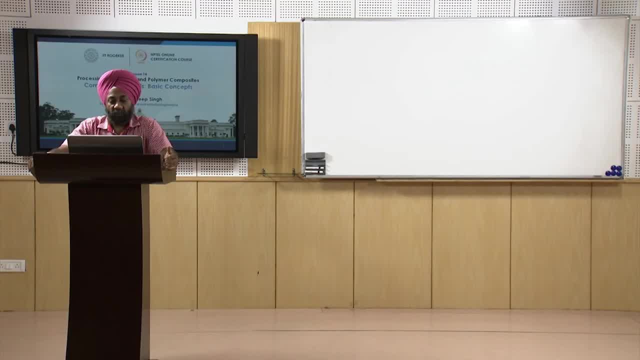 properties of the composite. or we can say the properties of the composite should be an improvement over the properties of the constituents. Last point: a manmade composite is usually produced by intimately mixing and combining the constituents. So, specifically, manmade is written because I have told you in the very beginning of today's 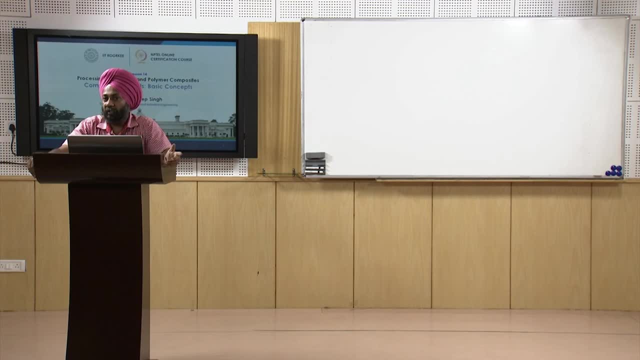 session that there are naturally occurring composites also like wood and bones. So a manmade composite, if we will classify any material as a composite, must have been made by physically mixing the reinforcement and the ah this thing, ah matrix together. So physically means we will combine them using a machine or using a setup or using a may. 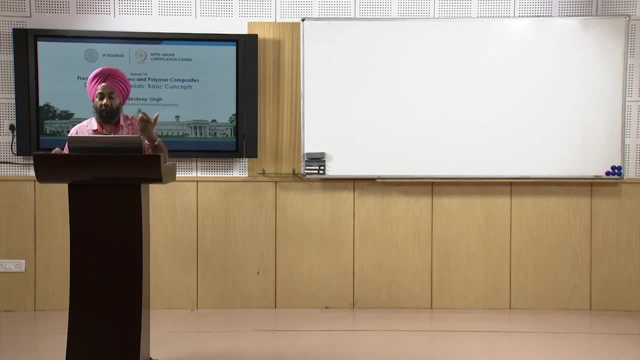 be: ah, physically, We manually, also by a manual labour, we are combining the reinforcement and the fibre together. So we will see there are different types of processes that are used for processing of composite materials and that we will see that what are the? some processes are manual, some 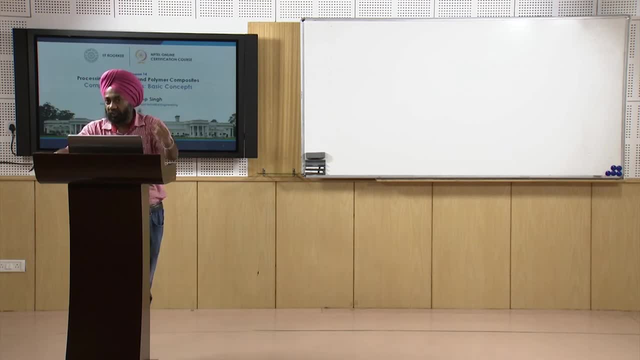 are semi automatic and some are fully automatic, and that is the major topic of our discussion, So which we will start in the next session with discussion on processing techniques for composite materials and we will see if some other introductory part is required. we will cover that also. 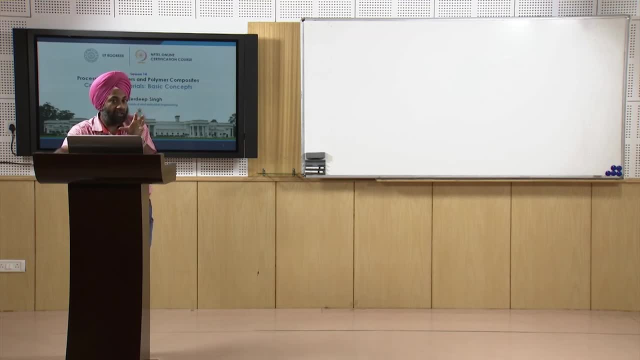 So now I think it should be clear that, how you will differentiate a alloy and a composite, how you will differentiate a polymer blend and a composite material. Now, very quickly, let us just see the different types of reinforcement. So, in case of synthetic composites which are manmade, composite, different types of reinforcements. 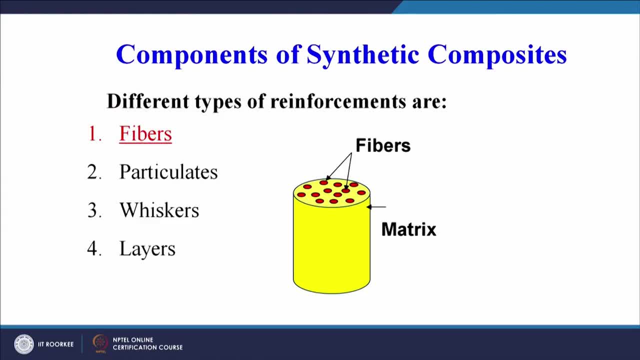 can be used. So on your screen you can see yellow colour is representing the matrix. the yellow colour on your screen is representing the matrix continuous phase and the red colour are showing the fibre tips. the fibres may be running all along the matrix. So this is one type of reinforcement. then particulate- you can see the yellow colour again is depicting.